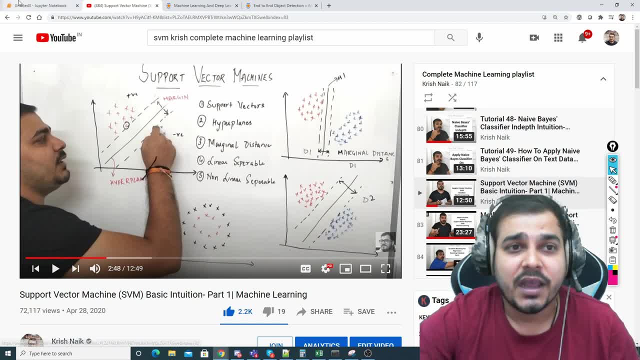 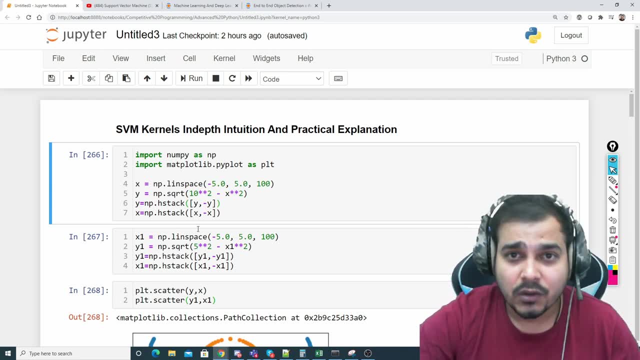 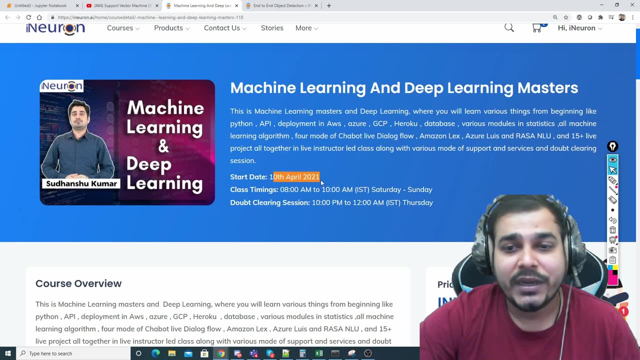 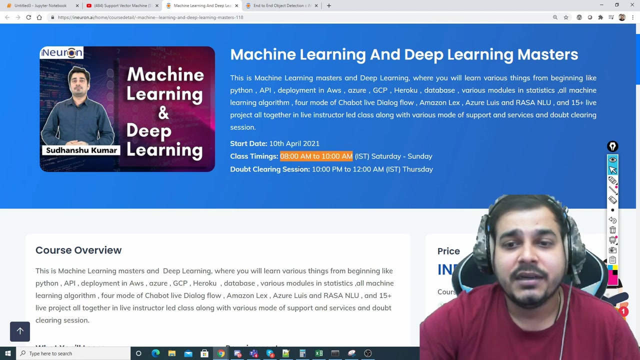 Now, this is very, very important. You just complete both this particular videos and then you probably start with this and let's begin the SVM kernel things. Before this, I just want to give a quick announcement because many people are asking about the affordable machine learning and deep learning course. So it is going to start on 10th April 2021.. Again, in this particular course, again, the class timing is 8am to 10am IST and the doubt clearing session will be 10pm to 12am IST on Thursday. Okay, and in this, this will be the entire course, So you'll be able to understand all the different types of kernels. So if you're interested in this, you can go ahead and watch the video. I'll try to explain in a much more simplified version. So if you're interested in this, you can go ahead and watch the video. I'll try to explain in a much more simplified version. So if you're interested in this, you can go ahead and watch the video. I'll try to explain in a much more simplified. 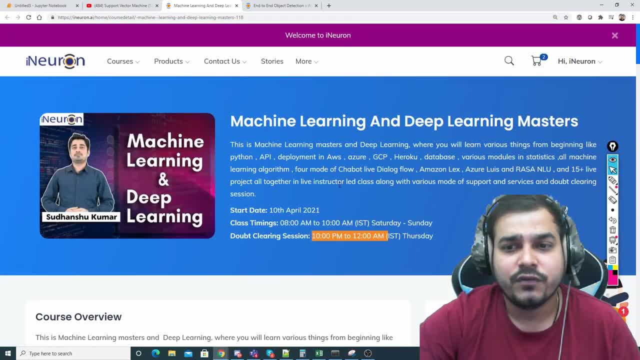 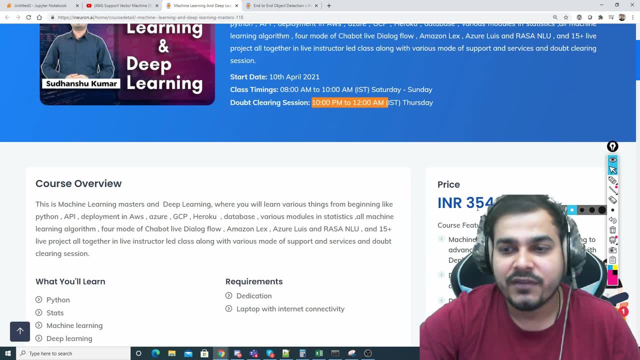 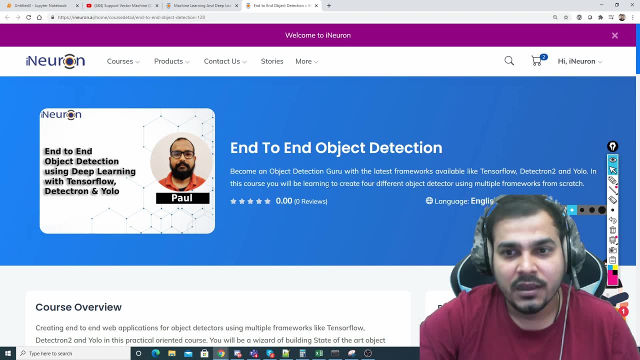 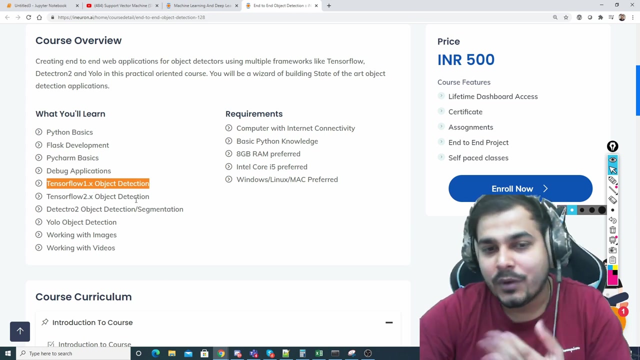 syllabus. here you can see how many months- probably four to five months, five to six months- it will take to complete this particular course. for you all It is the same affordable course, So the price will be 3540.. Apart from that, iNeuron has also started a self paced course which is called as end to end object detection. Remember, this is completely what all things you learn in this is that you'll be learning TensorFlow 1.0- greater than one point object detection. greater than two point object detection with different, different algorithms like RCNN, for example. 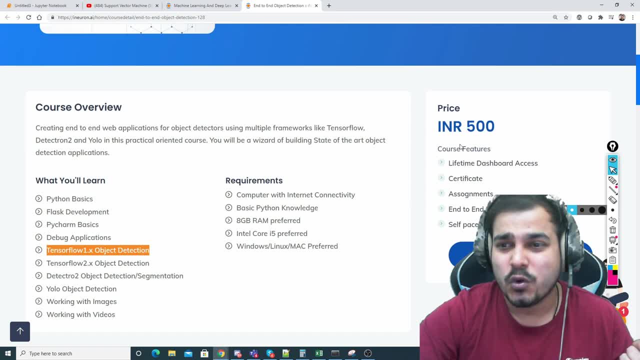 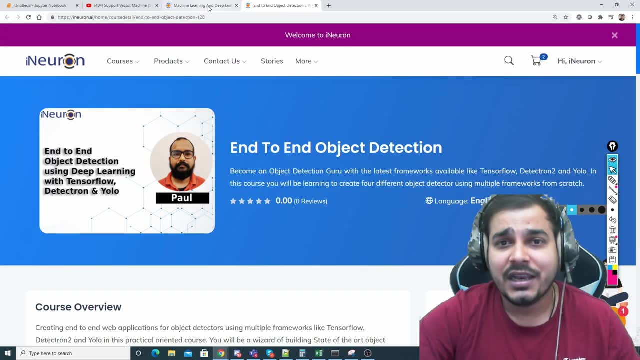 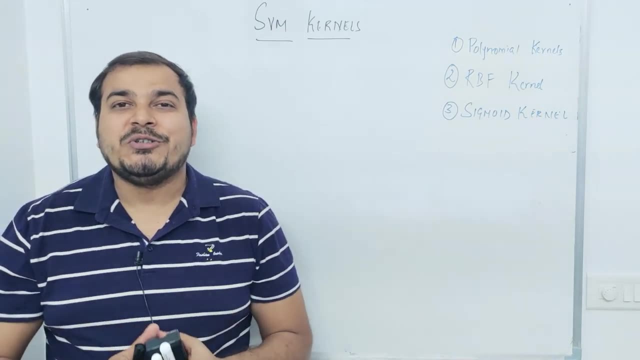 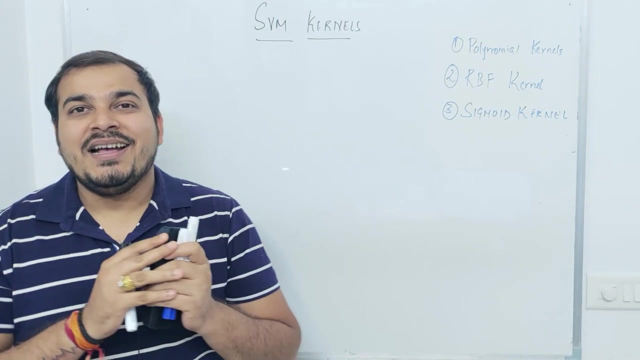 This course price is 500 and the content will be available for a lifetime. OK, So yes, just go through this. All the link will be given in the description. Now let's go back and try to understand what is SVM kernels. Hello, all my name is Prashnak and welcome to my channel. So, guys, it's been many days. I did not upload any videos with respect to Whiteboard. Definitely I also missed Whiteboard, But again, due to time constraint, I was trying to make a proper system set up and I was to upload videos. So for those of you who are interested in this course, you can go ahead and watch this video. I'll try to explain in a much more simplified version. Apart from that, I'll try to explain in a much more simplified version, But again, due to time constraint, I was trying to make a proper system set up and I was to upload videos. 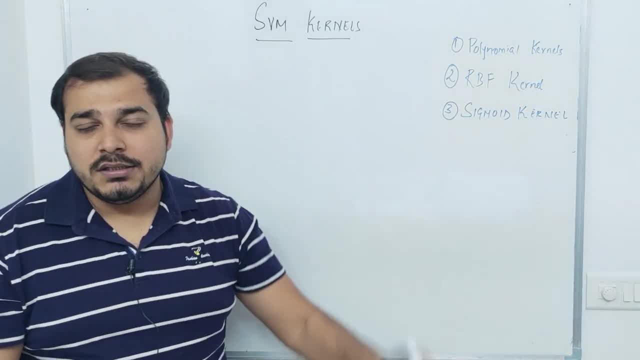 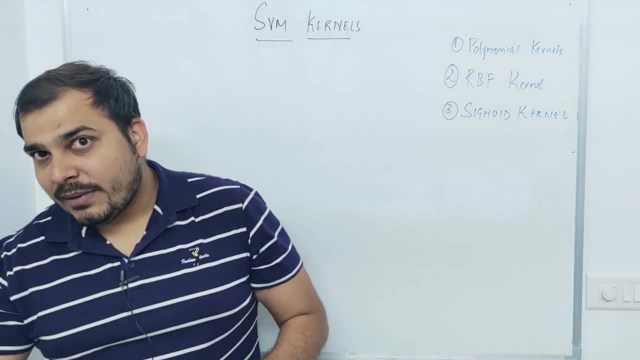 videos over there. so let me continue with respect to svm kernels. so in today's video we'll understand what this svm kernels is and, if you are following my complete machine learning playlist there i have already taken about support vector machines and the maths like how we usually used to. 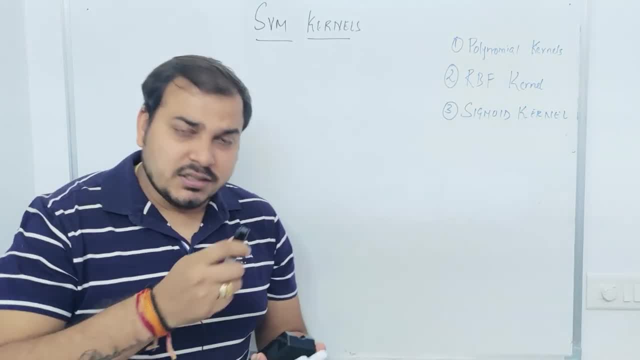 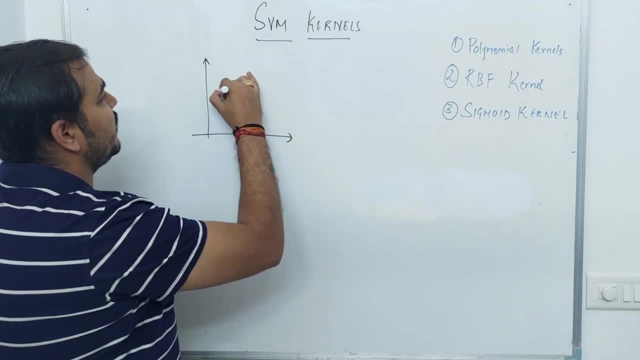 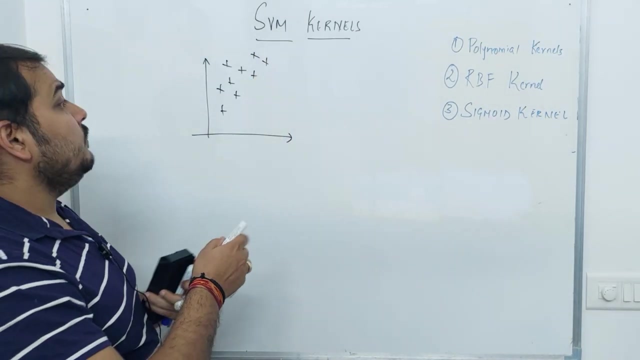 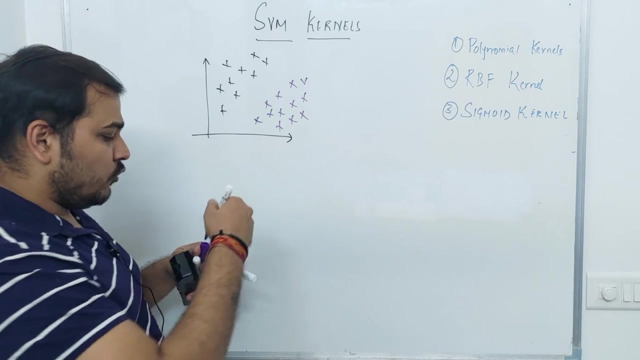 how svm actually works. we have understood all those things. just let me revise that specific thing, like with respect to svm. suppose i consider some problem statement like this a kind of classification problem, right, so suppose this is my classification problem. then, with the help of svm- suppose these are two classes- what i can do is that i can actually 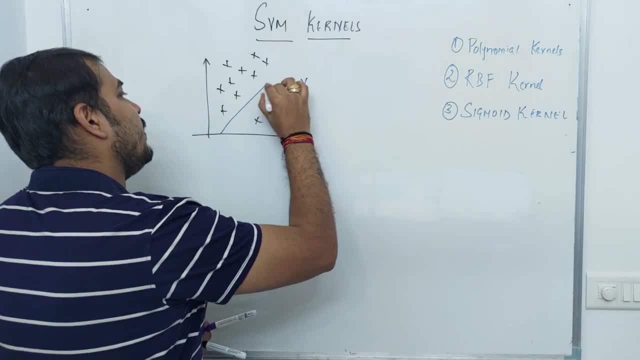 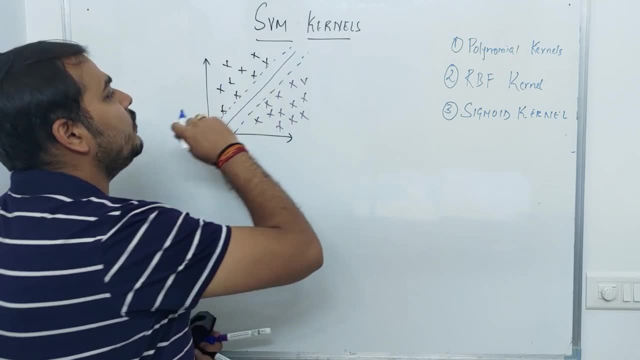 create a margin. okay, first of all, i try to create a hyperplane and top of it i can actually create a margin. okay, and with the help of this particular margin, we will be able to classify these particular points. now, whenever we try to create this kind of hyperplane and the margin there are usually, 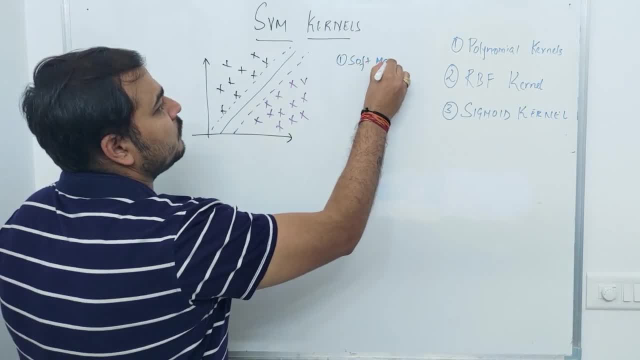 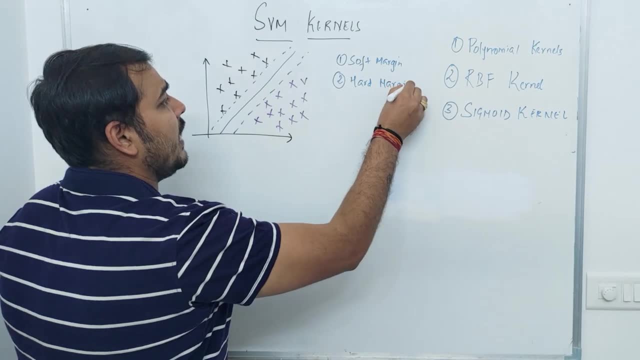 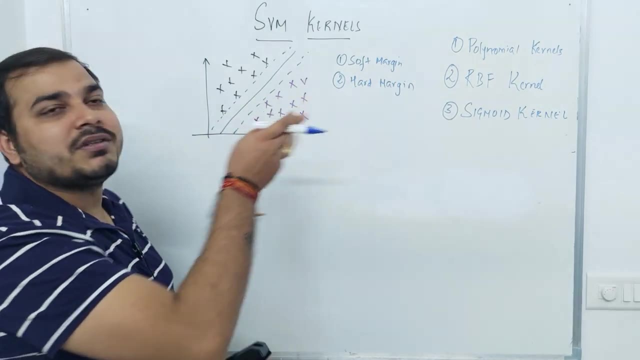 two types of margin. one is soft margin and the second one is hard margin. i think we have discussed about this. this example that i have been showing you is an example of hard margin, whereas in the terms of soft margin, you know there will be some percentage of errors. that basically means 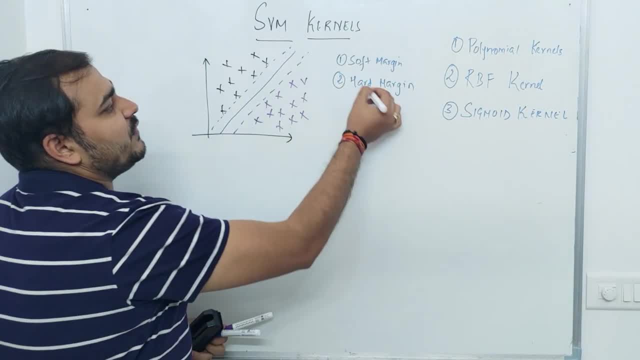 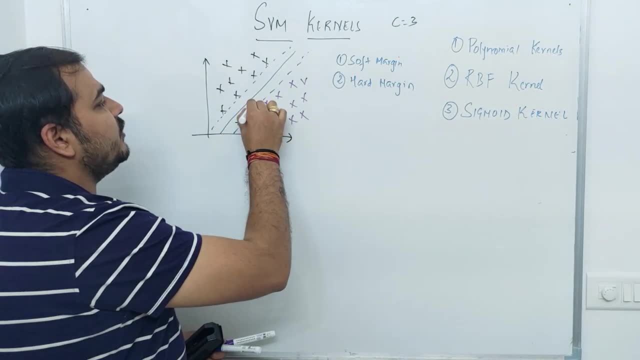 suppose this particular point gets indirectly classified. suppose if i say my soft margin has an error, of c is equal to three, this basically means that i can actually put three points over here. suppose three misclassification is happening. we can consider it that. okay, this will only be the hyperplane. 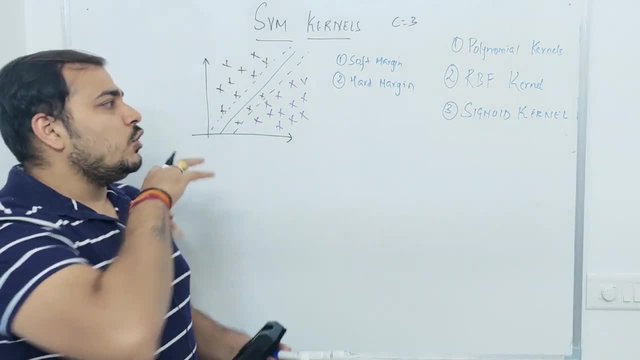 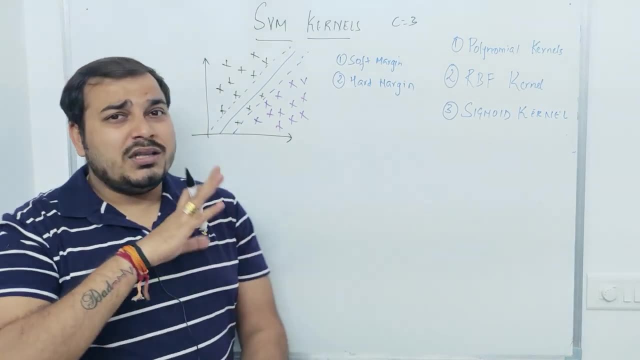 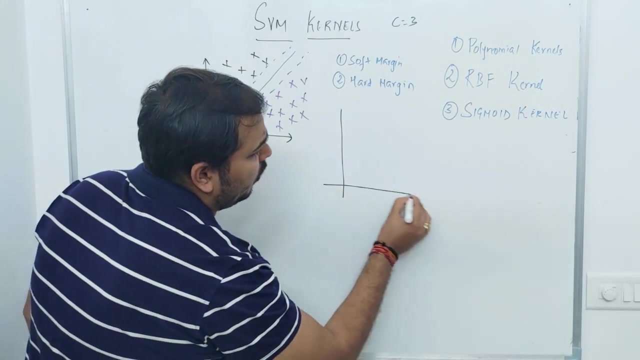 similarly this point. suppose three misclassified points are there. you know, we can consider that. so that is the basic difference between soft margin and hard margin. so we have discussed already all these things with respect to the maths implementation, with respect to everything, but still there is a question being asked about how do we know if a portion is linear or if there is a portion? 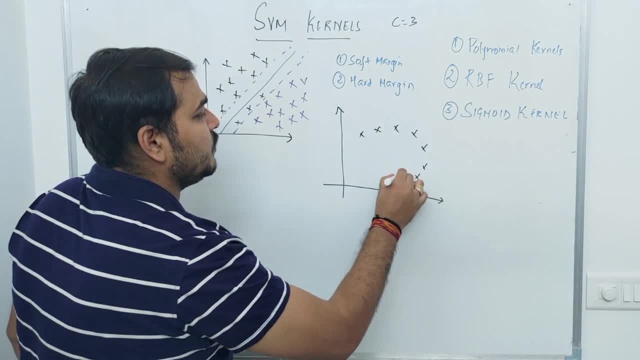 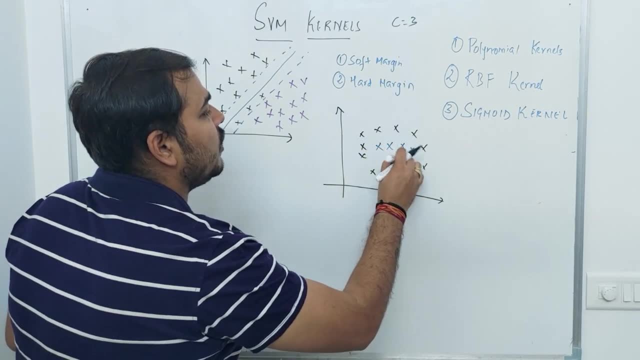 that is linear and if there is a portion that is linear. that is a very, very important question. what if i have a data set like this? suppose, if i have a data set like this which is not linearly separable, there is no possibility that this particular data set is not linearly separable. 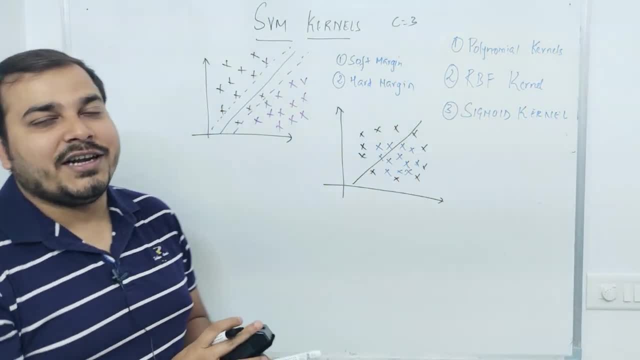 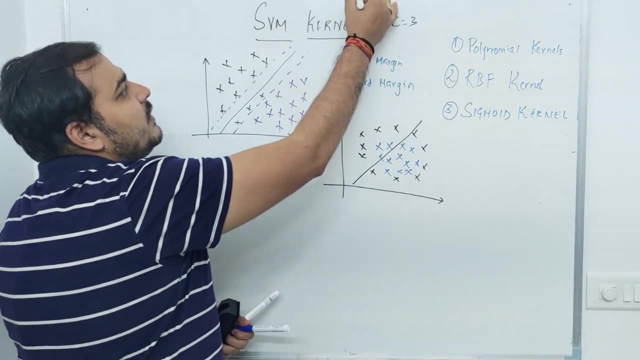 right suppose. if i try to draw a best fit line, then here you can see that the percentage of error will be definitely increasing. so in this particular scenario, what can we do? you know so that I told you that we will be using this SVM kernels, and they are different types of SVM. 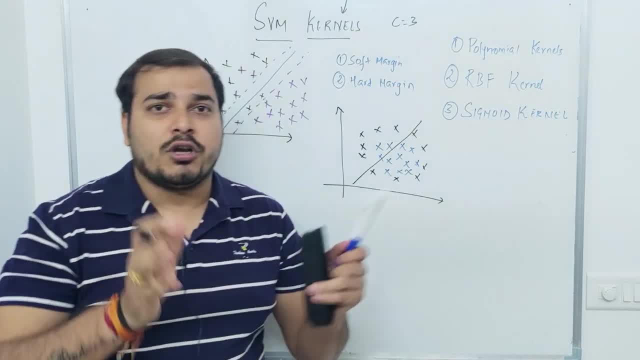 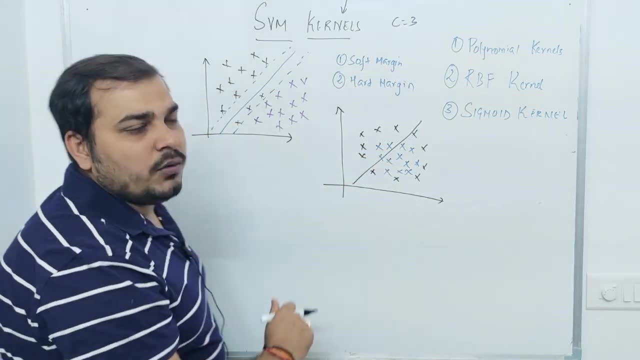 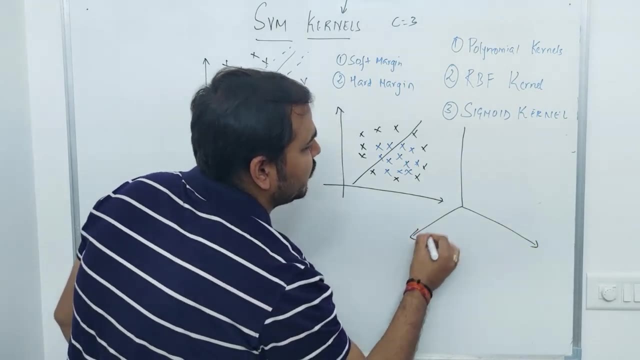 kernels, polynomial kernels, RBF kernels, sigmoid kernel and many more kernels. So we will try to understand. how does this SVM kernel work? So, in short, in this particular scenario, suppose, if I try to apply an SVM kernel, what this will do is that this will convert this into from two dimension into three dimension. 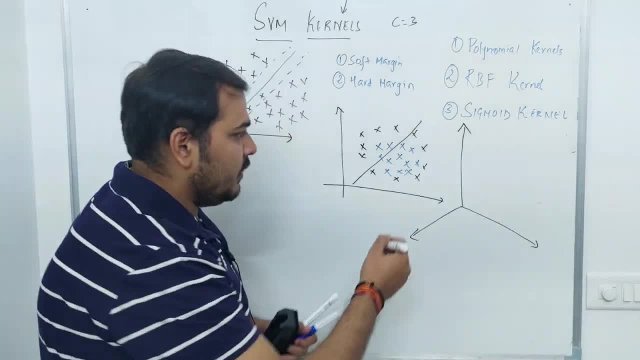 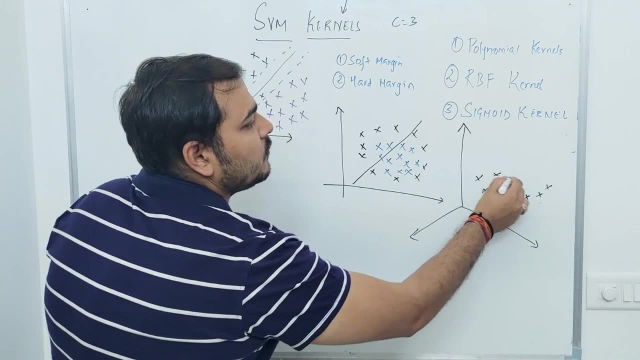 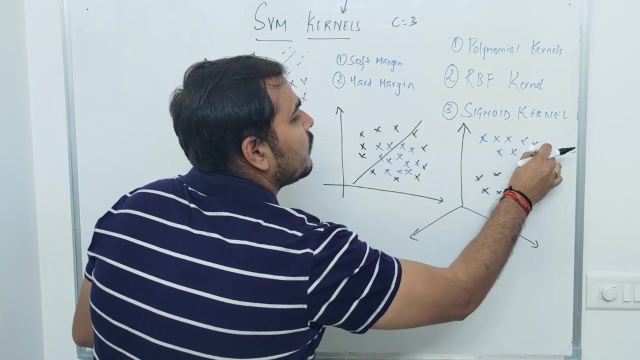 and then this middle points. probably this will be first of all. the below points will be somewhere here. okay, just taking as an example. okay, and the middle points will be raised over here. okay, and we will try to create an hyperplane over here for the. 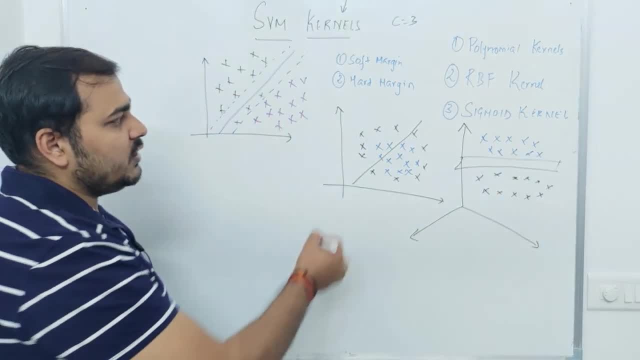 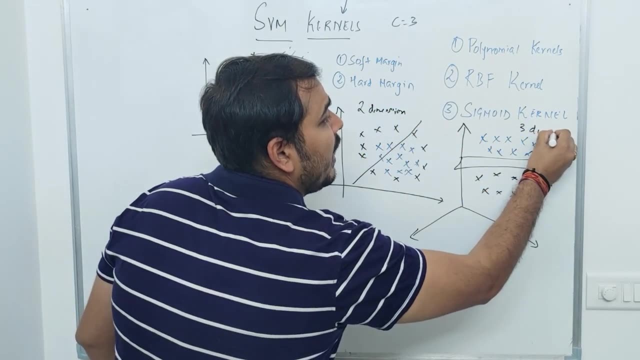 division purpose. okay, So this is what it is going to do. it is basically going to convert a two dimension- in this particular example, two or three dimension, and probably create a plane in order to separate this particular plane. So, in short, what does SVM kernel do? 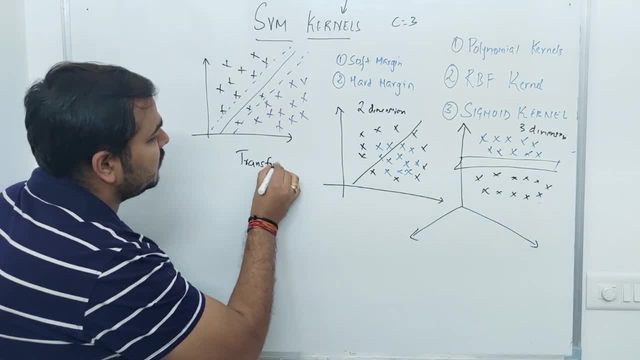 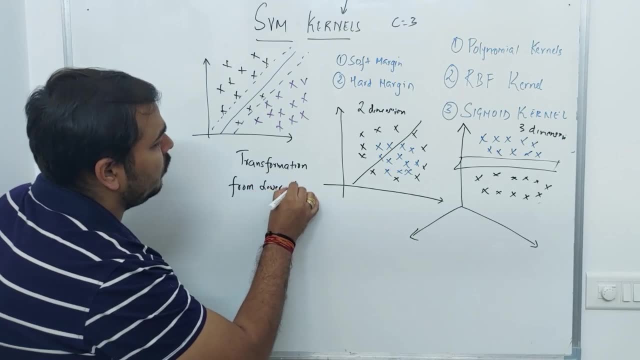 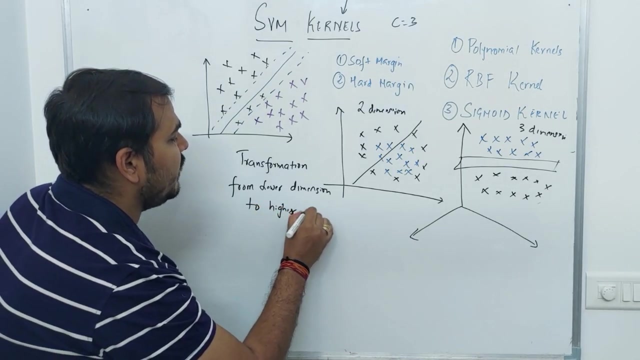 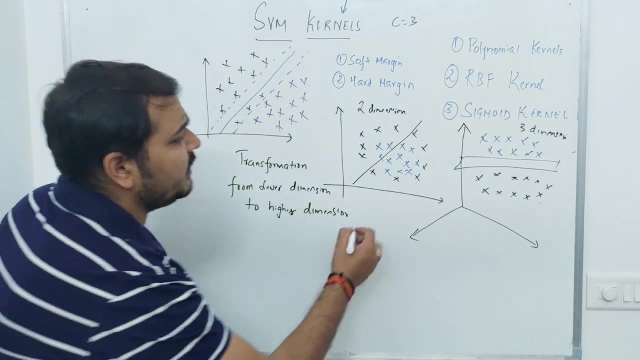 It does some kind of transformation. it does some kind of transformation from lower dimension to lower dimension, to higher dimension, right, higher dimension. Now the question arises: how does it does this kind of transformation? It does it with the help of some mathematical. 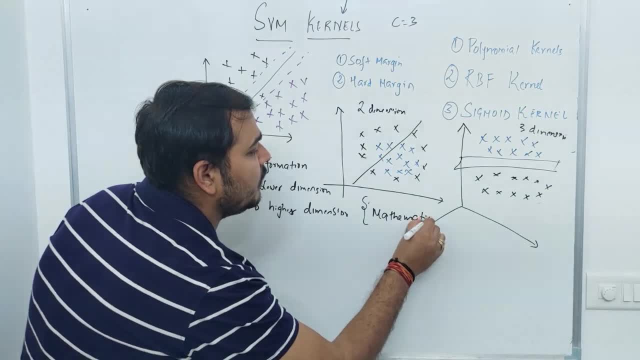 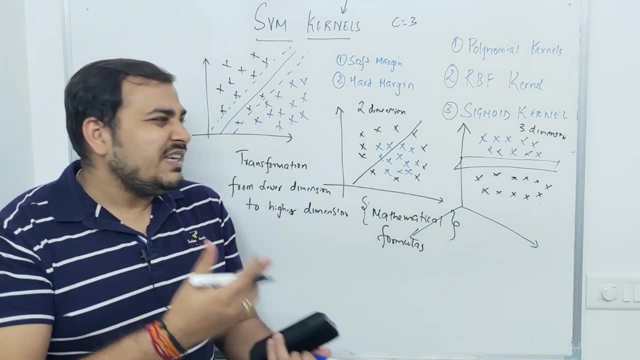 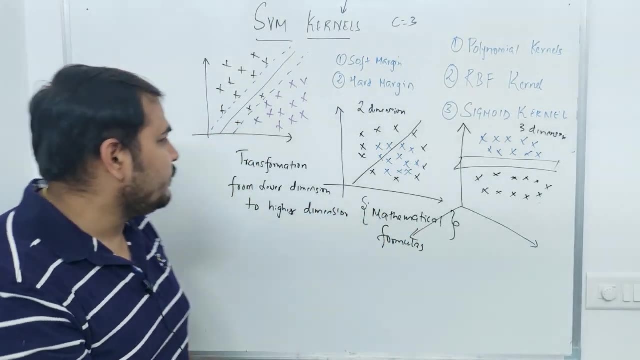 Formulas, okay, mathematical formulas- very simple, okay. I will try to make it much more easier when I am trying to explain you. with respect to SVM kernel, the thing is that it will try to use some kind of mathematical formulas and then it is going to convert this. 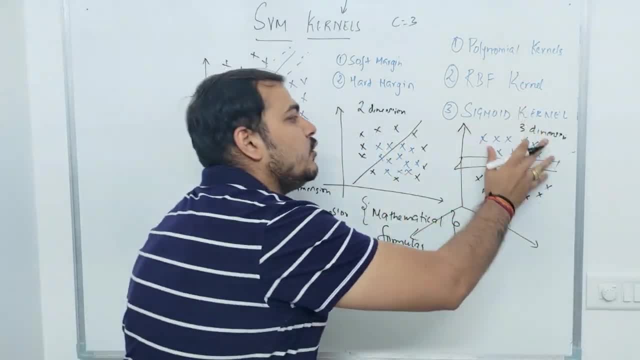 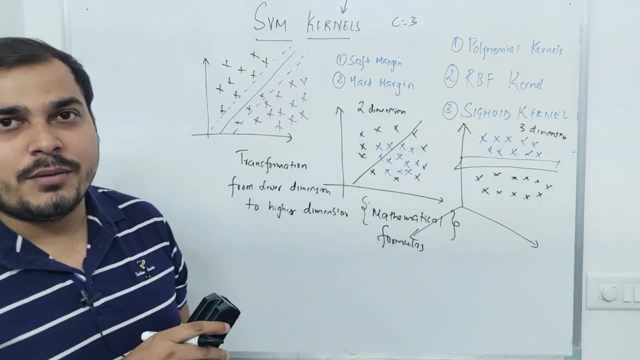 lower dimension into a higher dimension, and then it will be able to split this particular data or classify this data with the help of hyperplane. okay, so let us understand what is this mathematical formula. I will try to understand some of the examples, so before that, I will just drop it and remember. 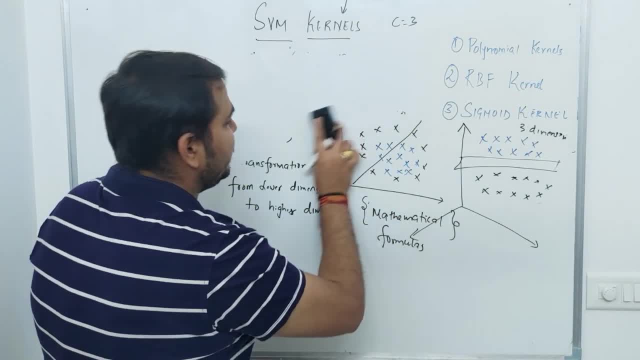 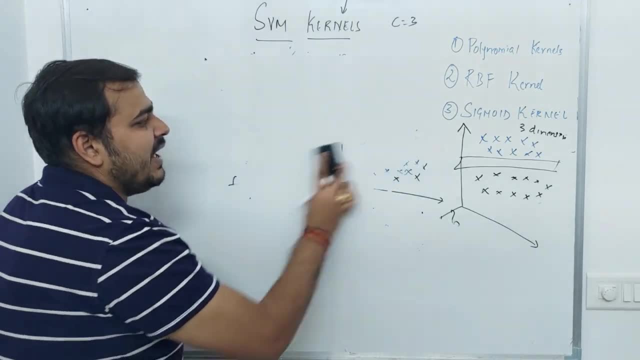 guys, as I said, okay, there are some math formulas, which is basically converting this lower dimension into higher dimension. it does not mean that you really have to by heart all the equations- and probably do it- but you just need to understand one working. so 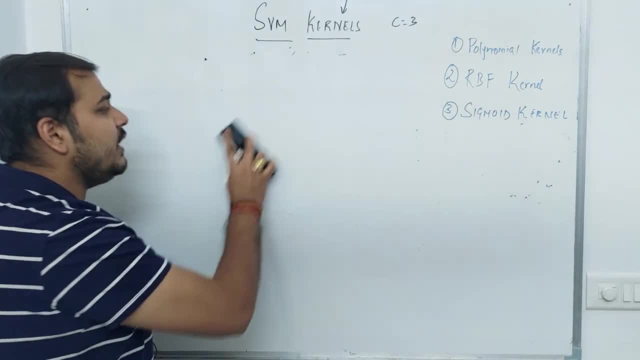 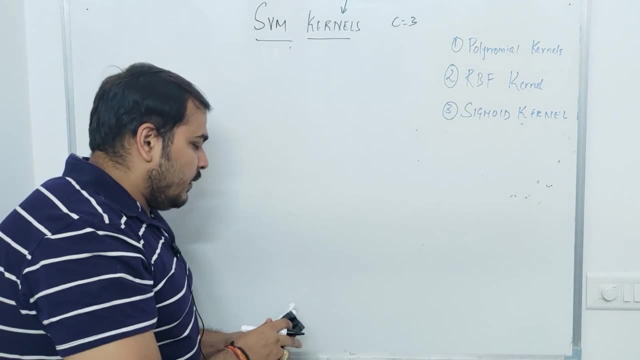 in this particular example, I will be showing you about polynomial kernels, and this will give you an entire example of how does polynomial kernels actually work. So okay, now let us see. Okay, So let me take one use case over here. suppose I have this particular. let us consider a. 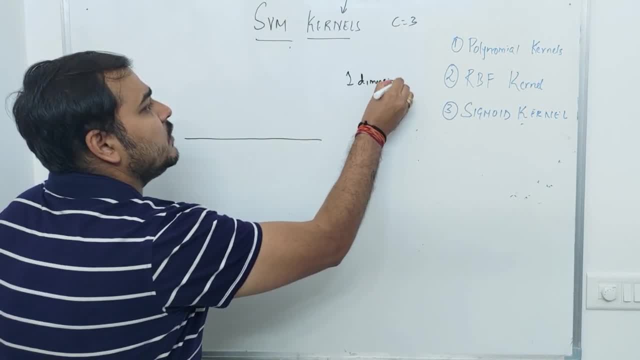 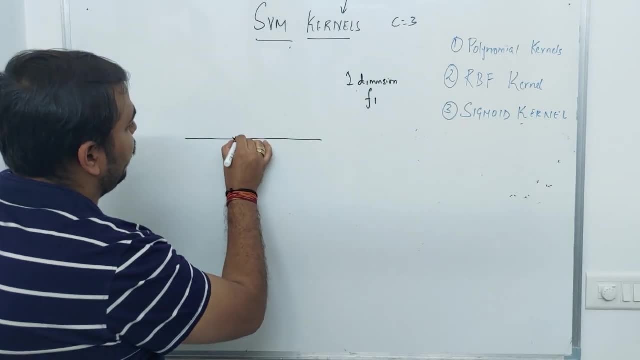 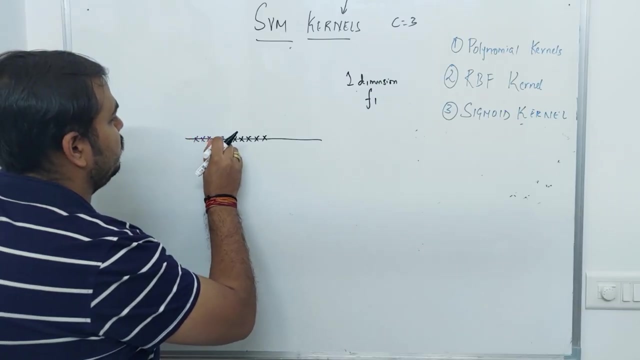 one dimension, one dimension points, suppose in this one dimension, suppose I have a feature one inside this I have two categories, suppose okay. so here are my some of my points, okay, and then I will try to draw some of the points here. 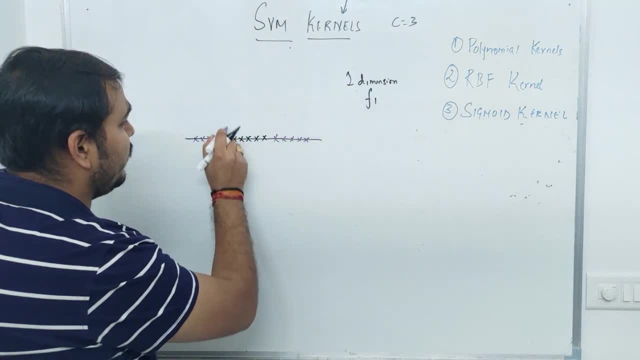 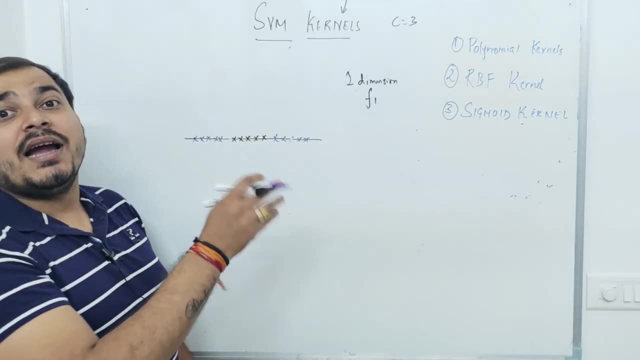 Now suppose, if I really want to classify these two points, I can either create one hyperplane over here, but again the error will be very, very high. here also I can create a hyperplane, but again error will be very, very high, in order to classify this particular thing right. 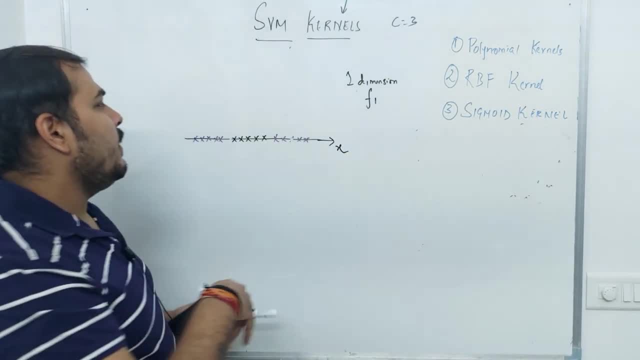 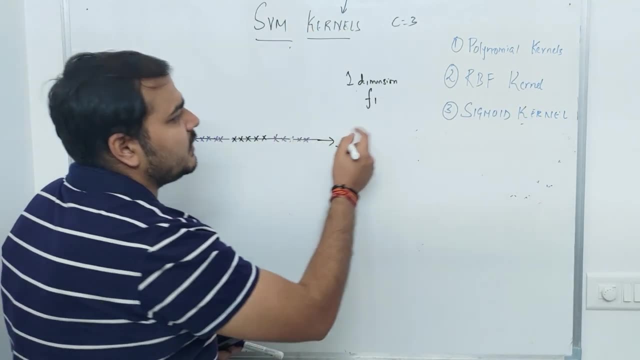 Now suppose, just consider that this is my feature x. okay, now the thing is that, since everything is lying in the same line, how do I use an SVM kernel so that I convert this one dimension into two dimensions, and then probably I will be able to, you know. 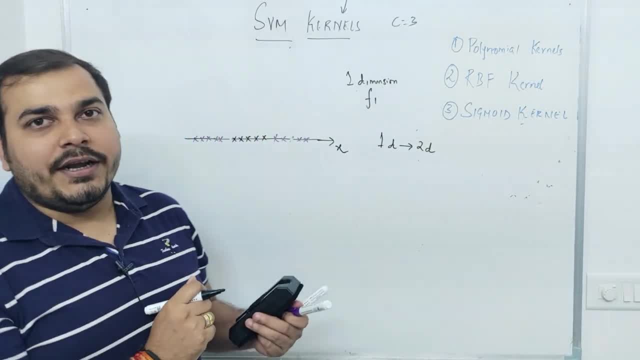 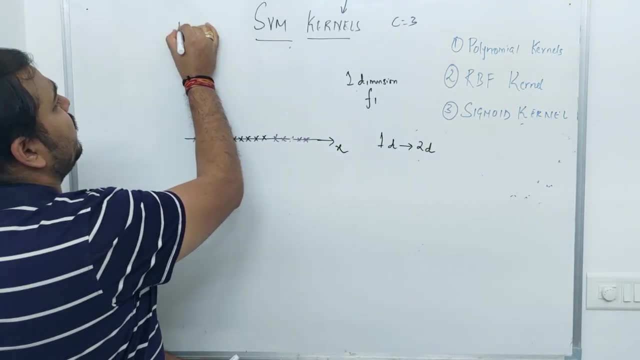 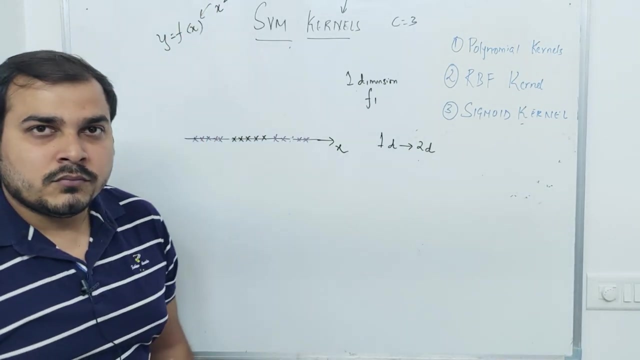 us probably draw a hyperplane And try to split this particular data or try to classify this particular data. So suppose I take this x over here. let me consider an equation: f of x. okay, y is equal to f of x and probably this function is nothing but x square. okay, and let me just put some. 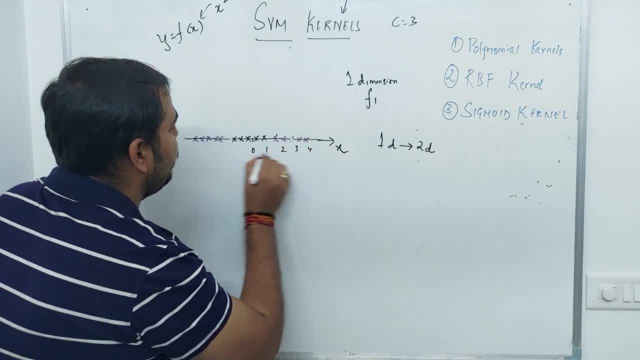 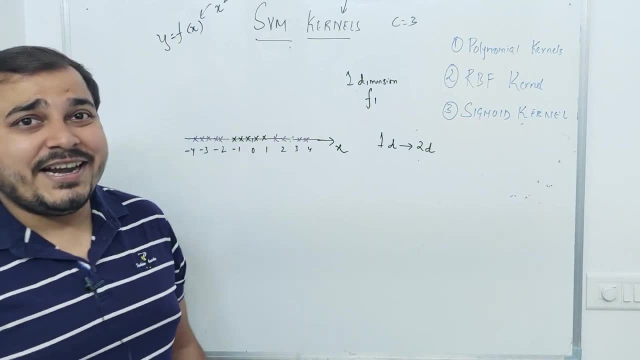 of the points. so suppose over here is 0,, 1,, 2,, 3,, 4, and here it becomes minus 1,, minus 2,, minus 3,, minus 4,. okay, so I have just mentioned it. it is zero centric data I have. 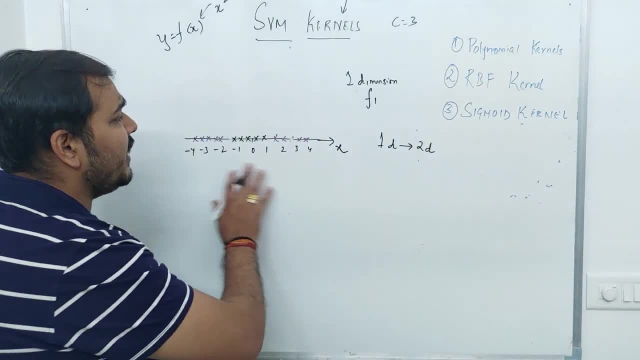 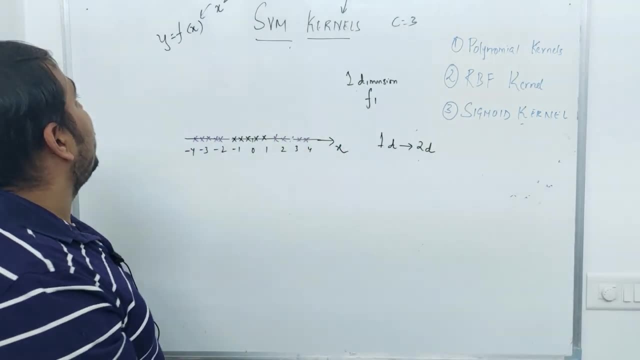 probably done some kind of a test, Some kind of transformation or standardization, so that I am making it with: mean is equal to 0, and probably standard deviation as 1, and I have all this particular data set. Now, when I do this kind of transformation, now, see this with respect to each and every. 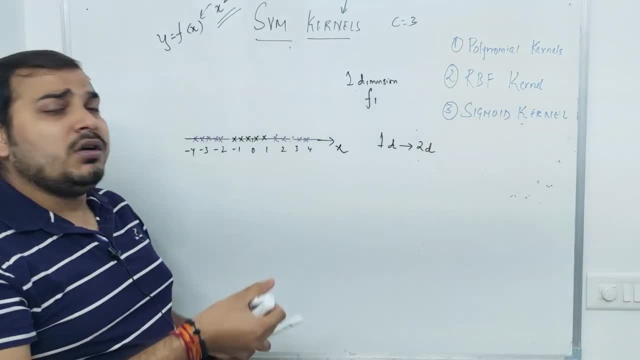 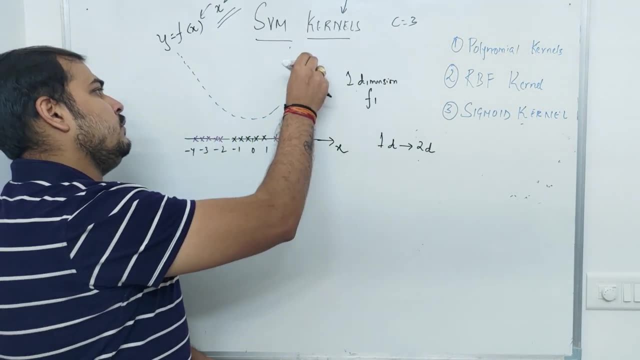 element. we will try to square it Now. when we try to square it out, probably what will happen is that we will be falling, forming this kind of curve, this kind of curve, right. so here we are, forming this kind of. 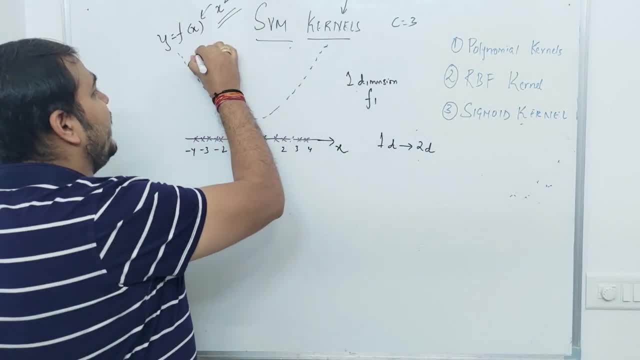 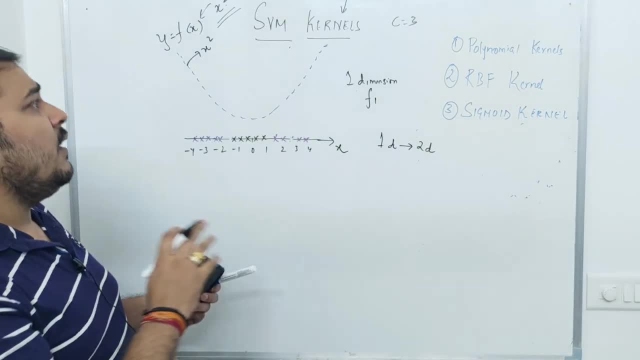 curve. Now what I have done. I have just created x. x is equal to x square, so I have applied this formula on this entire data set. so I have done this kind of transformation Now when I do x square, so I get this kind of parabola. after this, what I will do: I will. 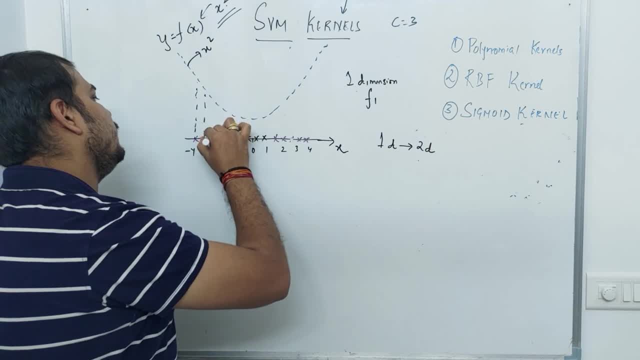 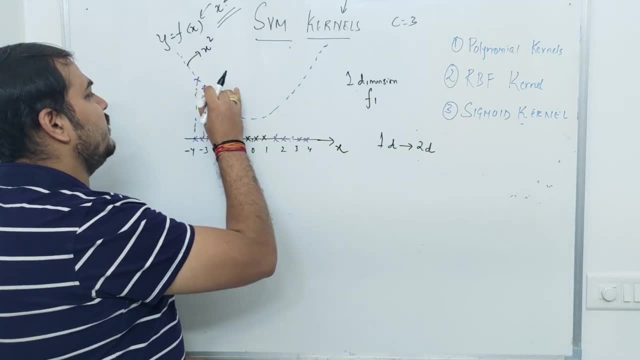 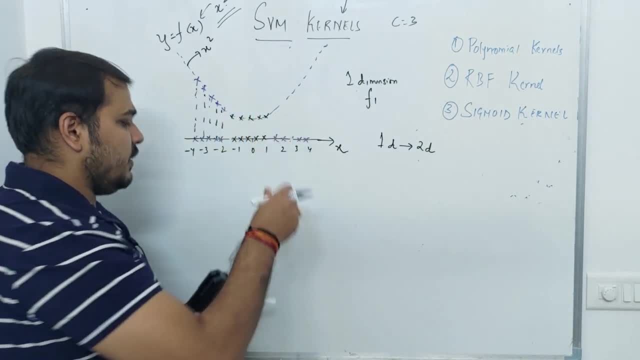 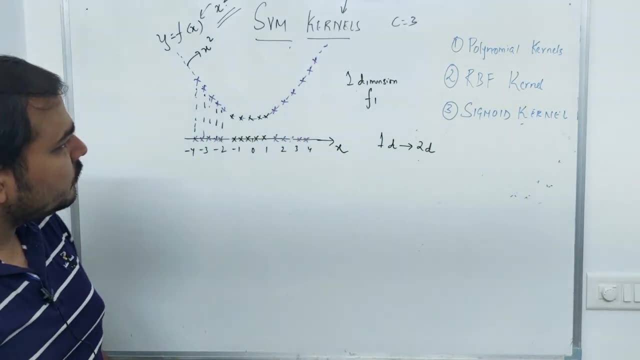 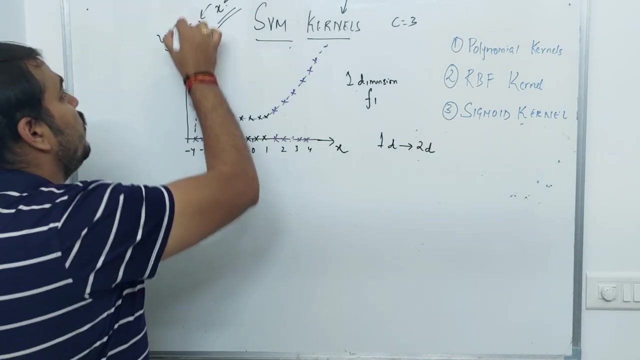 my this point getting projected, okay, and again after this, I have this kind all points getting projected here. Now you see this in short, what we have done over here by just equation, equating this particular equation. see, this x square is basically my y axis. now right, 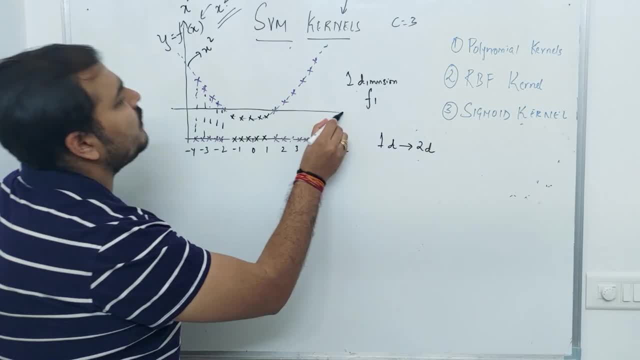 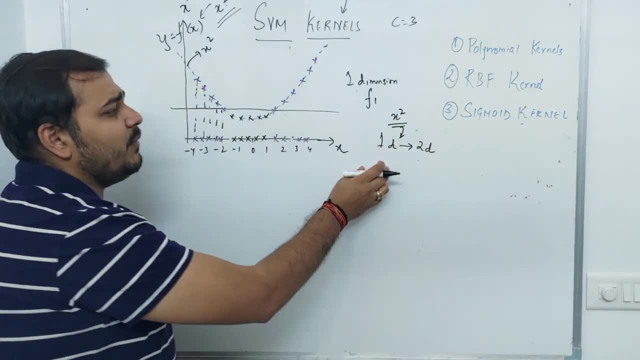 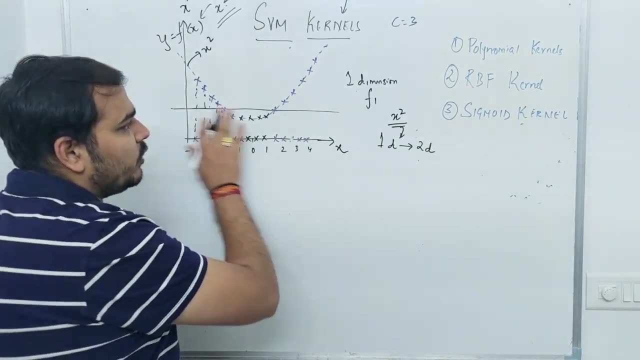 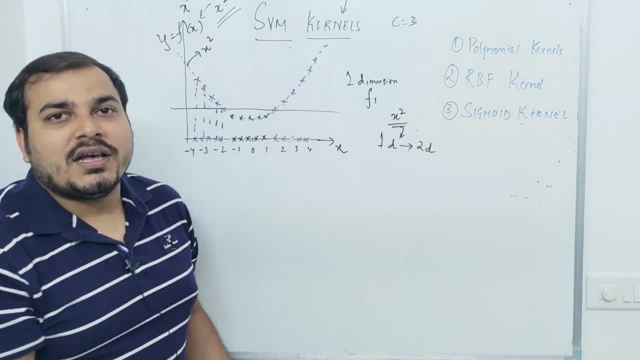 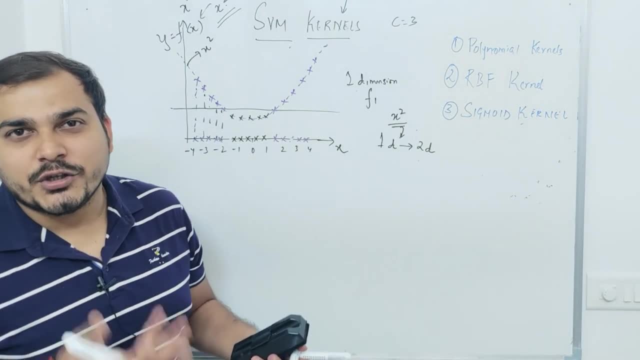 a small, you know this best fit line, basically the two classifier things. okay, This is what an SVM kernel is actually doing. Suppose, if you have a two-dimensional data, it will convert it into three. if they are three-dimensional, you can try to convert into four, probably into five, probably into. 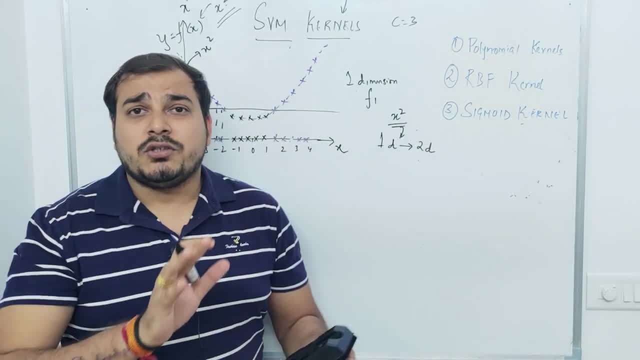 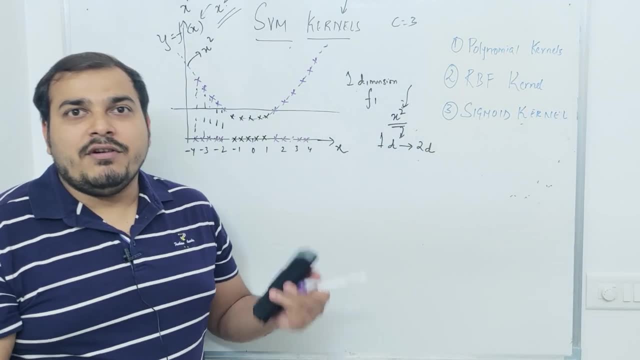 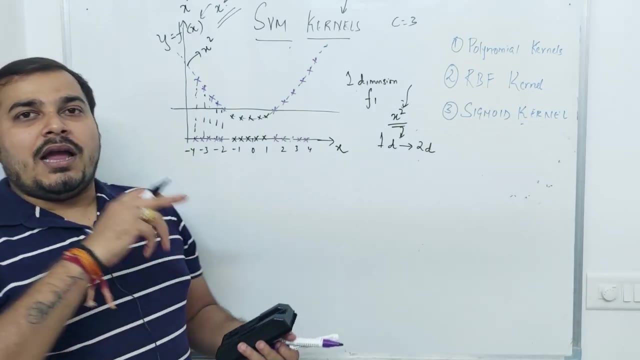 this is the simple thing that is doing, but how it is doing is this mathematical equations- what all complex mathematical equations will come that we will try to understand again. I am not going to discuss about every mathematical equation. probably in the next session after this I will show you a practical application with the help of polynomial or RBF or sigmoid. 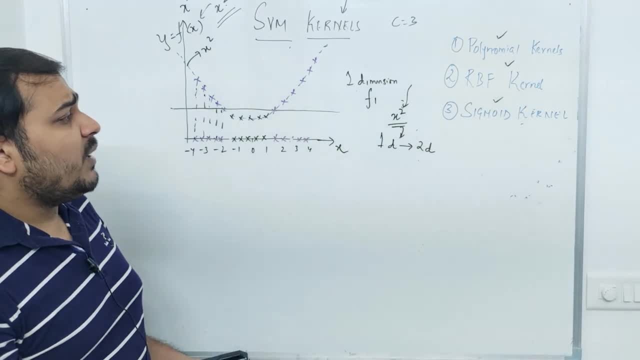 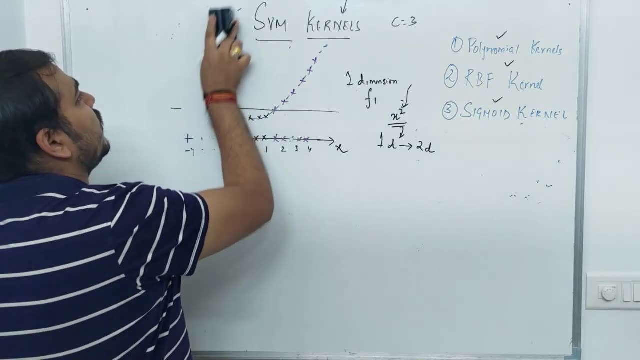 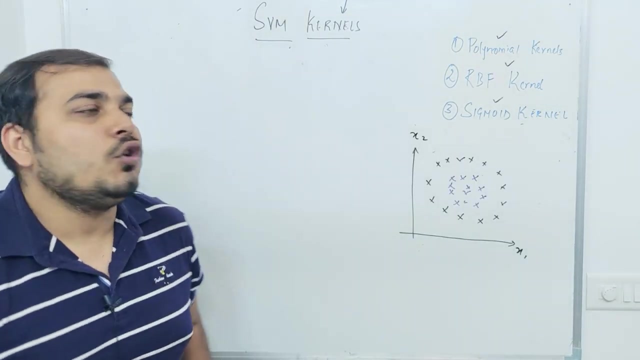 right, we will try to cover this three. let us see what will happen, but before that, let us take an example of polynomial kernel. so again, I am just going to rub this, ok, and then we are going to understand with respect to polynomial kernel equation. ok, ok, guys. so let 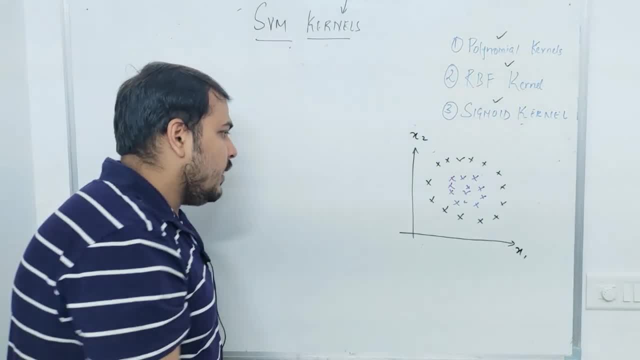 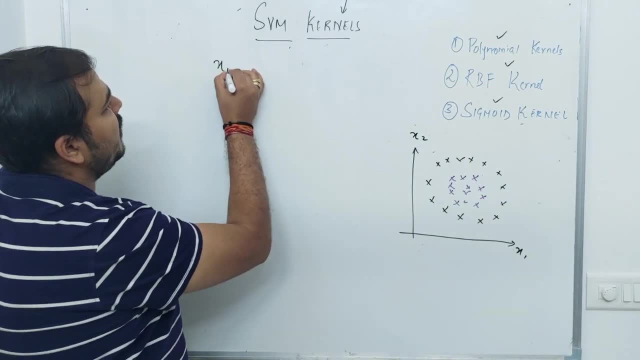 us go ahead and understand about polynomial kernels. ok, let us consider that I have a feature- x1 and x2- which looks like this in a scattered plot. so in my data set, what I have, I have x1, x2 and I have my output variable y. consider that this belongs to 0. this belongs to 1. so 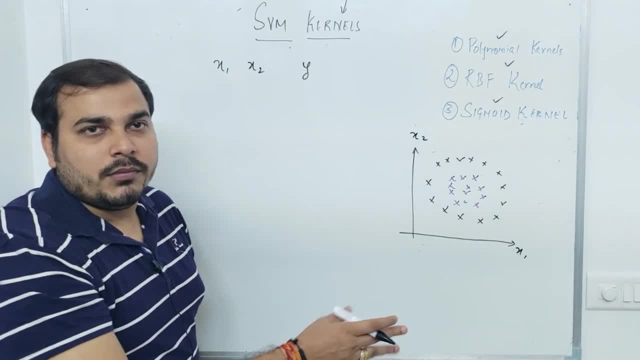 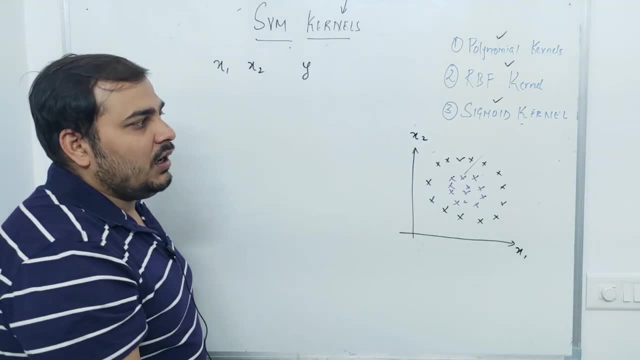 this is x1 and x2. ok, now I know that in this particular problem if I try to apply a linear regression always remember first you have to check this. apply SVC normally with the kernel linear. linear basically means that just try to draw a straight line there probably. 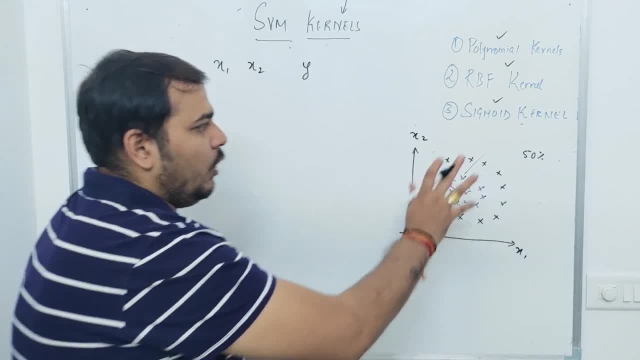 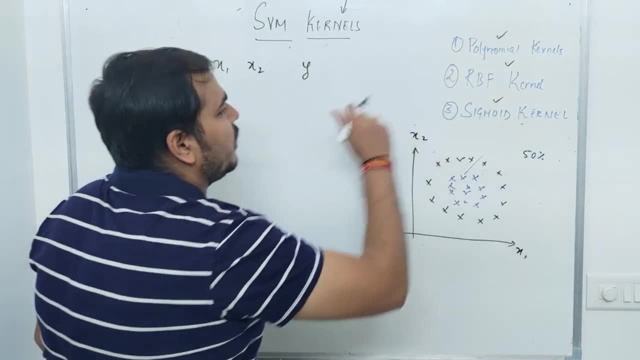 the accuracy will be near 50%. okay, now, when we see this kind of problem, the next step is that we have to apply SVM kernels. ok, let us consider about polynomial kernel. polynomial kernel formula looks something like this: we can say that it is a polynomial kernel and. 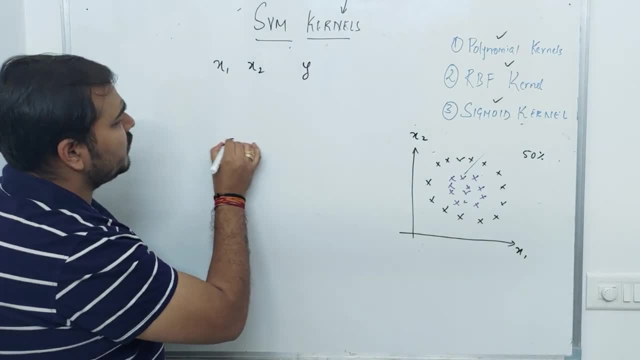 the formula is something like this: we can say that we have to apply SVM kernels. ok, now let us see what is the polynomial kernel. so here we have a kernel for the polynomial kernel. Suppose I will say polynomial kernel is equal to. there will be an operation which is like: 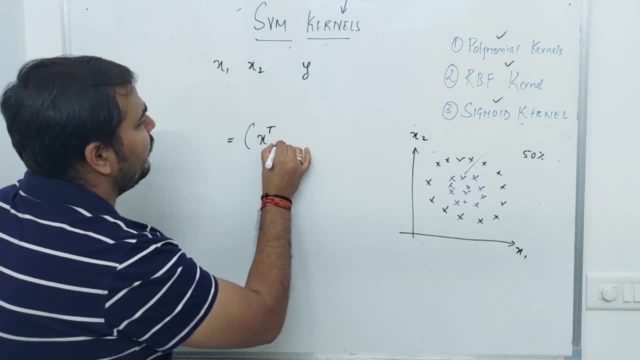 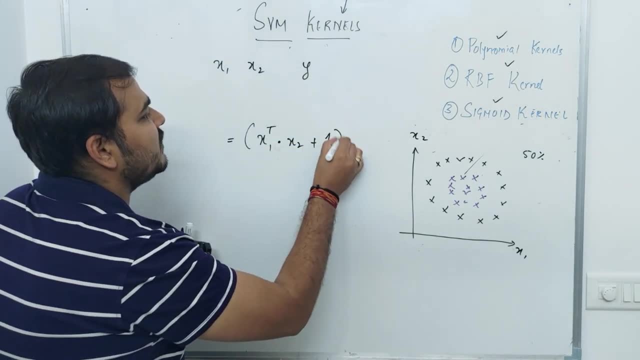 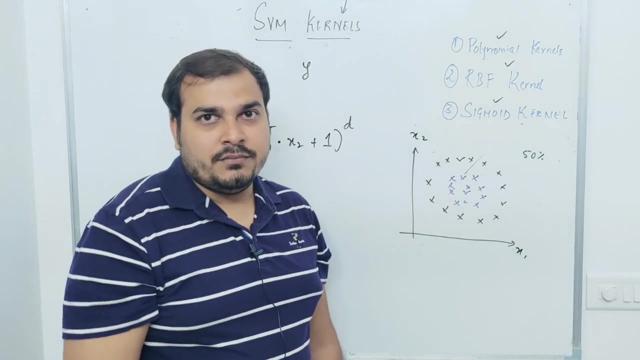 this x transpose of 1 multiplied by this will be a vector operation. vector operation of x, 2 plus 1, which is an identity matrix, and d is basically the dimensions. In this particular scenario it is two dimensions. probably we want to work with one dimension. 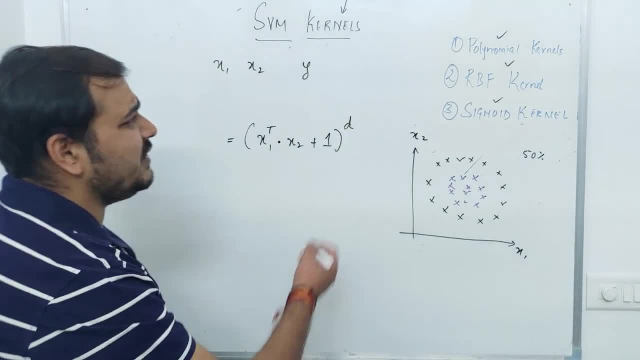 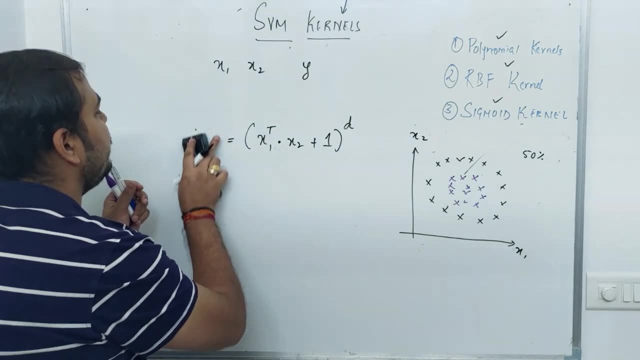 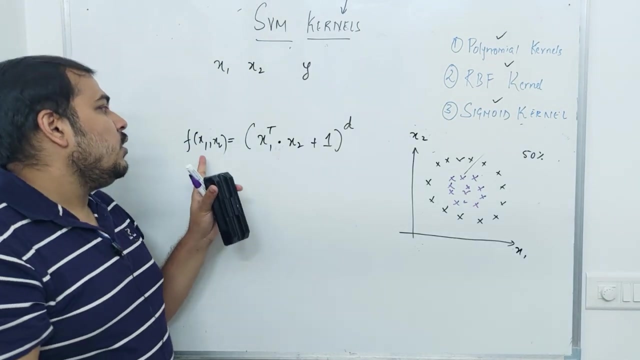 so just consider d as that specific dimension, and this is a simple formula of polynomial kernel. I will say it as pk, or let me just write it down over here as f of x. f of x 1 comma x 2.. So I can write it as: f 1 comma x 2 is nothing but x transpose. t is the vector operation. 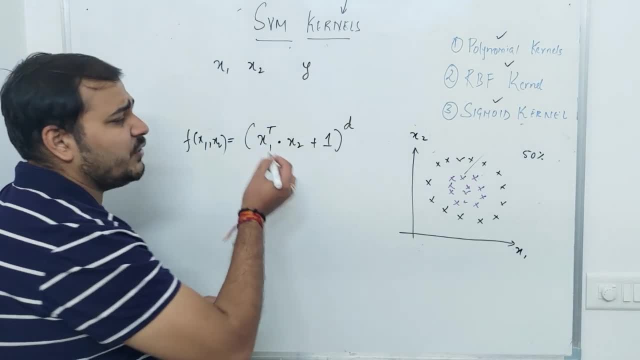 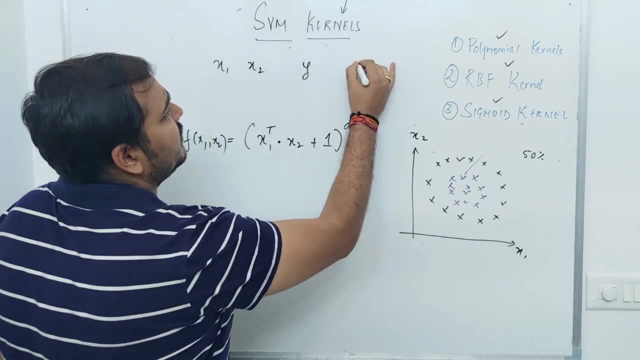 with respect to, basically, multiplication vector operation with respect to x 2, now, remember, when I have a data set, x 1 comma, x 2 is nothing but x transpose t, this is represented by the x2, I can basically write this y as function of x1, x2, right, very simple, just a function. 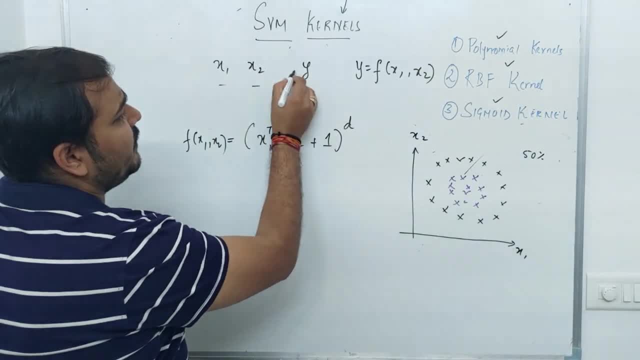 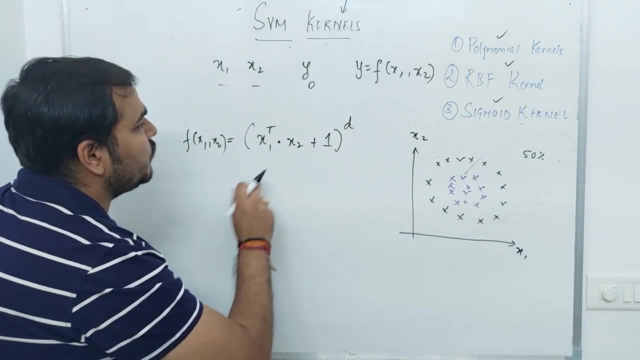 of x1, x2, because x1, x2 are my independent feature and, based on this, the value will be either 0 or 1, okay, Now, when I consider this particular operation, when I have to do this transpose operation, this transpose operation, will happen something if my data. 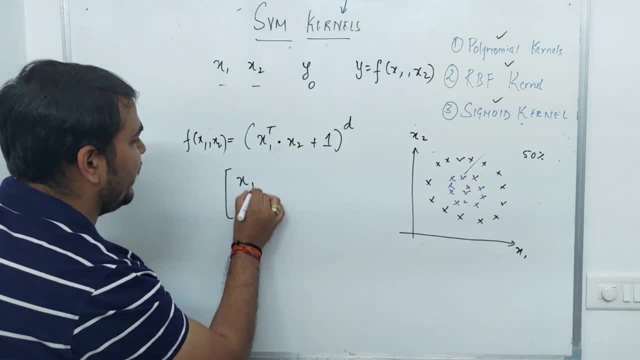 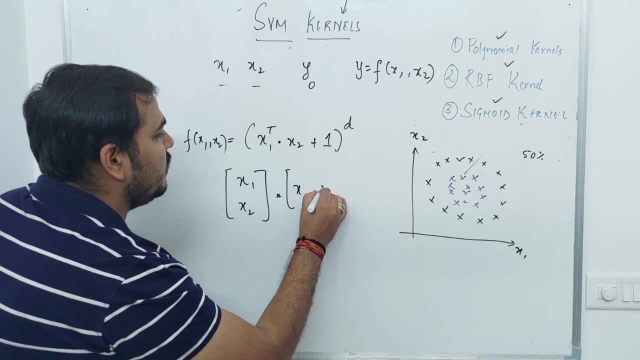 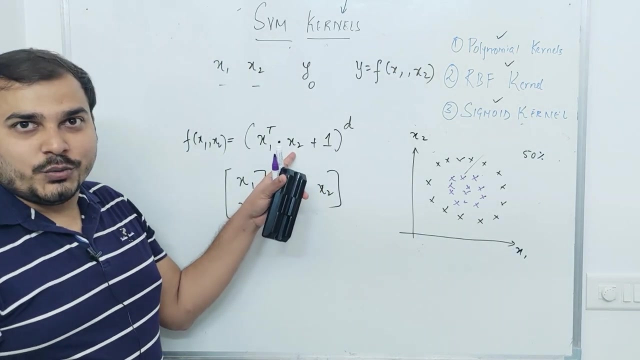 set is given like this: So I will be having x1, x2 over here, because x1, x2 transpose becomes like this: right, then it becomes a dot operation of x1, x2, okay. So this is the simple thing over here. because you may be thinking: then what is x2, right, just consider. 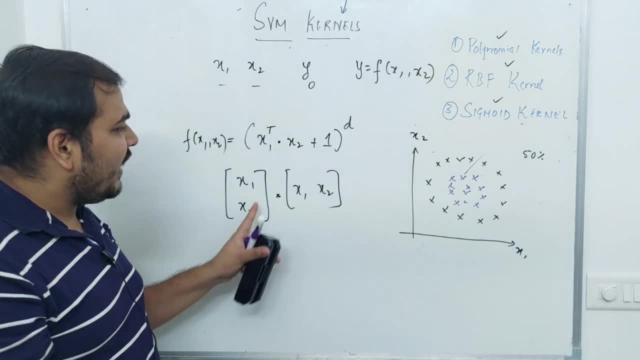 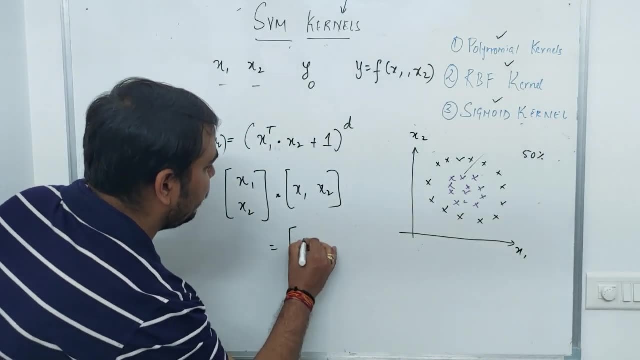 that if I have given a data set like this, I use the same thing and try to do a dot operation with the transpose of it. okay, Now, when I do this kind of operation, the first one will come as x1 square. the second one will come as: see this multiplied by this. right then? 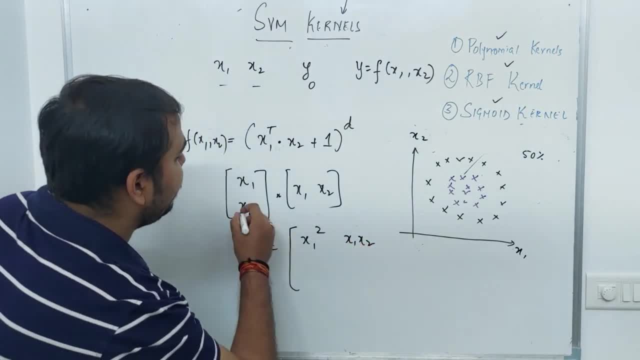 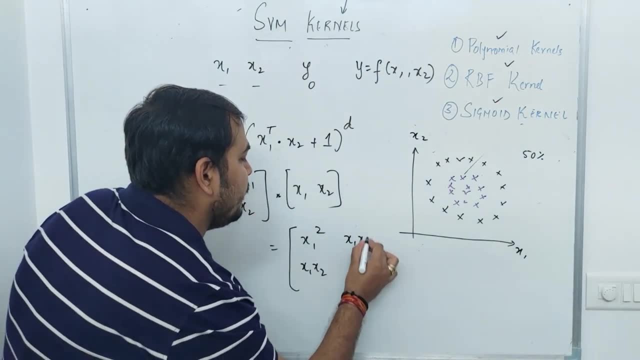 this multiplied by this. So I have two integers: x1, x2, then again I have x2, x1, x1 and x2 again, and then I have x2, whole square. Now remember one thing, guys: what I am getting over here. these are the 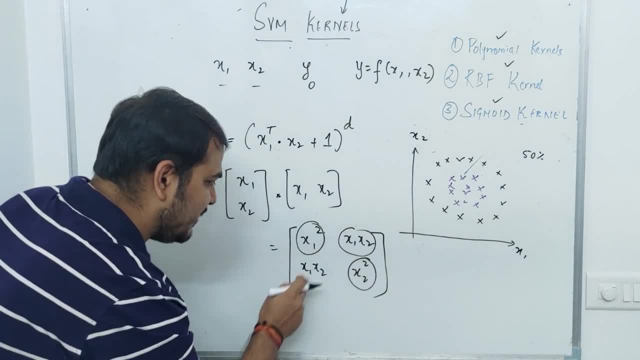 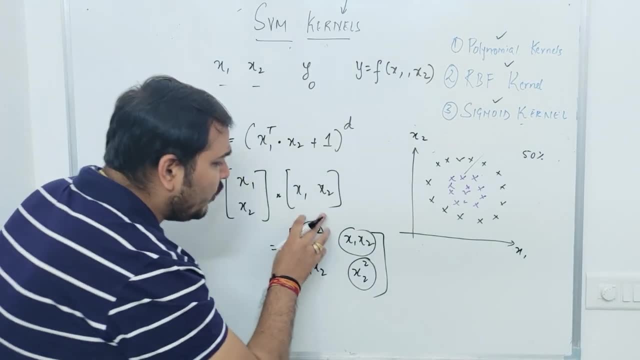 important components that I need to find out. Remember, these are repeated features, right? x1, x2, x1, x2 is also there, right? So I am just going to take the unique elements like x1 square, x2 square, and x1 and x2, right, I am going to take this entire thing, See. 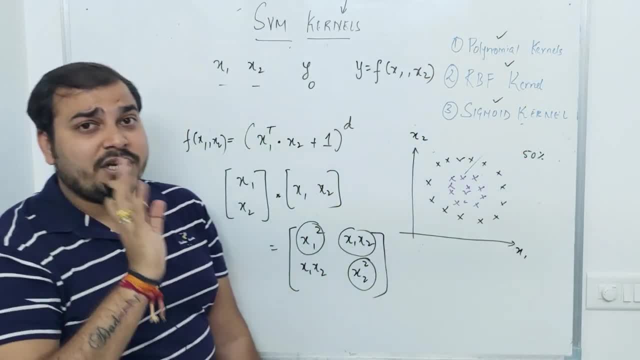 I am telling you how to do it right, so I am just going to take the unique elements like this: So how does the coronal operation happen? the polynomial coronal operation happens. this is the formula with respect to this. okay, After this, what I will do is that this: 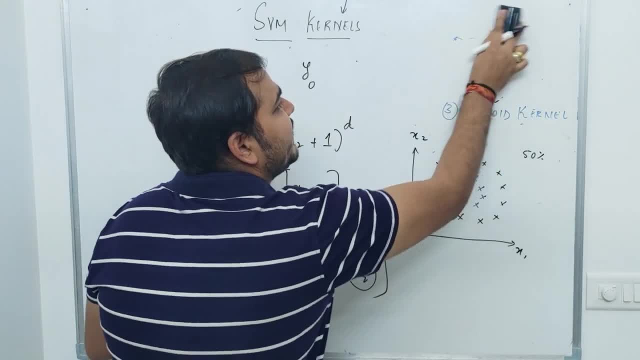 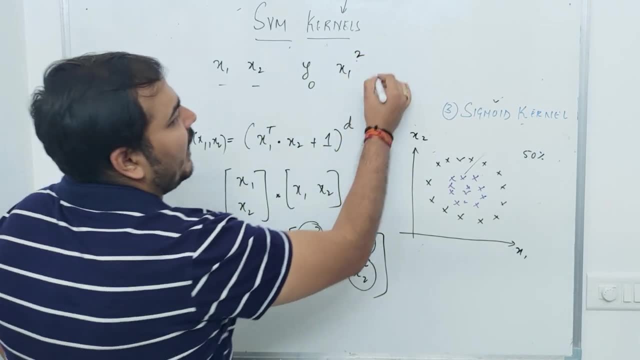 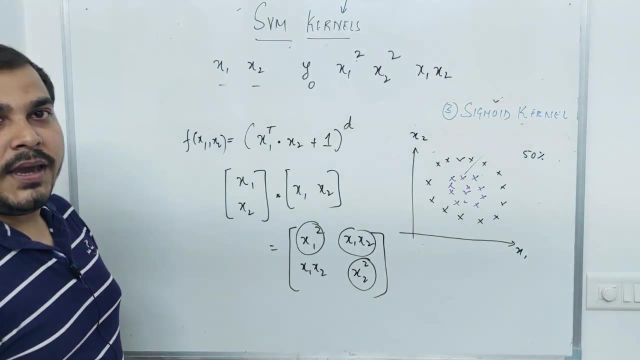 y will be like this: the next element that we probably need to find out is basically x1 square, x1 square, Then I need to basically find out x2 square, because this is the unitary, and then, finally, I need to find out x1, x2.. Okay, Remember this: two dimension points. 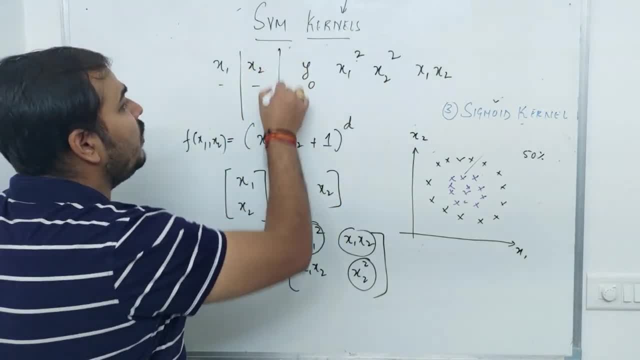 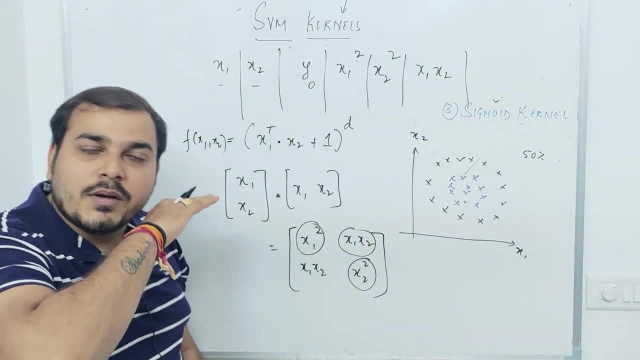 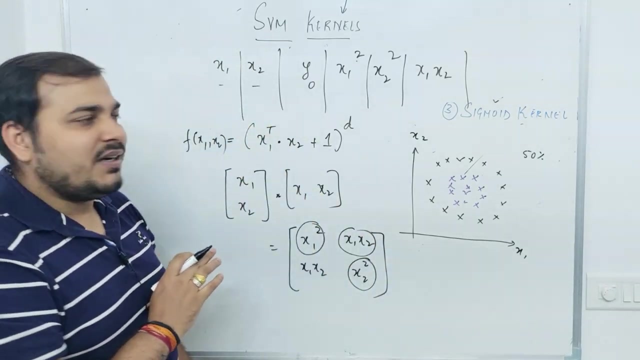 are becoming five dimensions. so these are my all the features now which I will probably using in order to convert this into a higher dimension and probably create a plane line. okay, again, with respect to this, I cannot just show you visualization in some other dimensions, but just understand that if now, if I 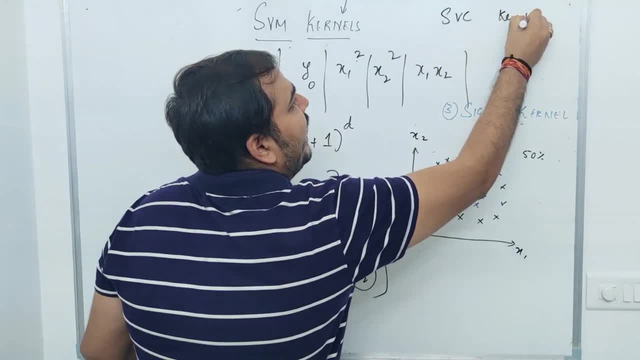 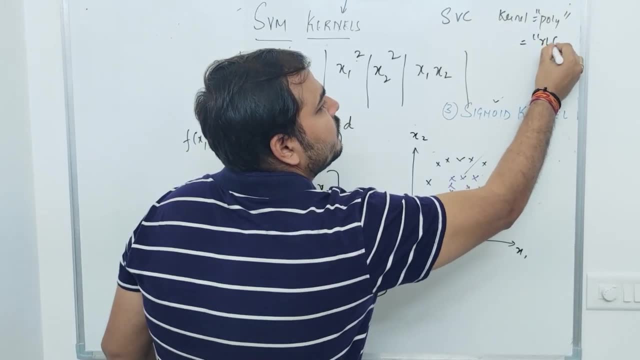 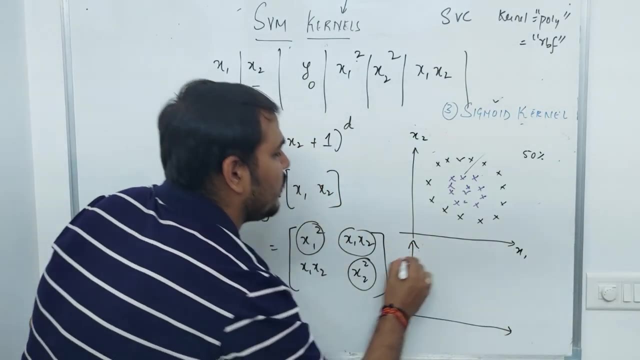 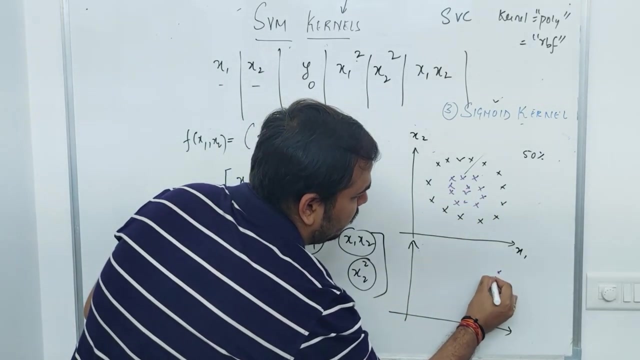 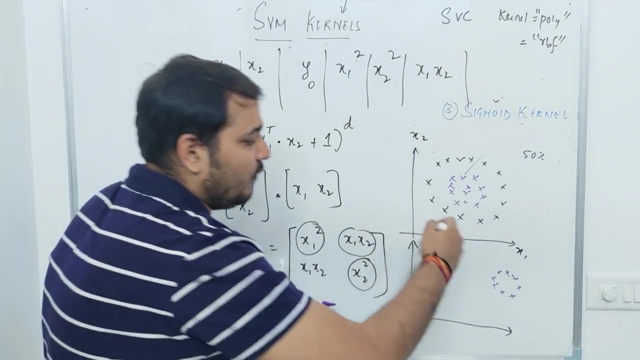 train my SVG model with kernel as poly. poly basically means polynomial, okay, polynomial or RBF. remember now this points that you see over here: this will become something like this. okay, this will become something like this. so suppose I take this and then this black point when it is getting converted into a higher 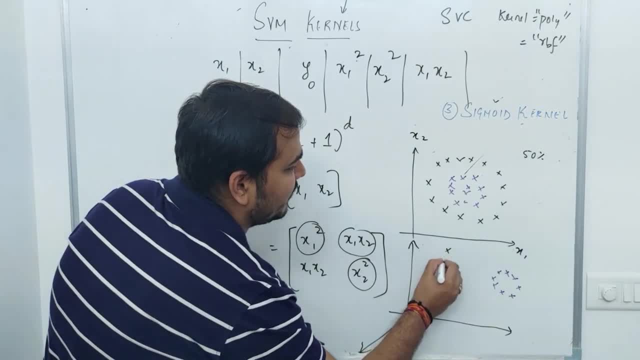 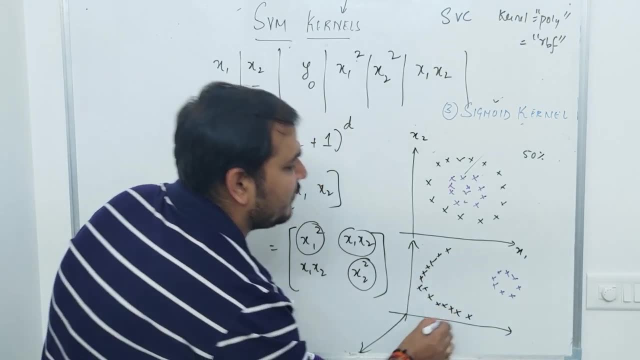 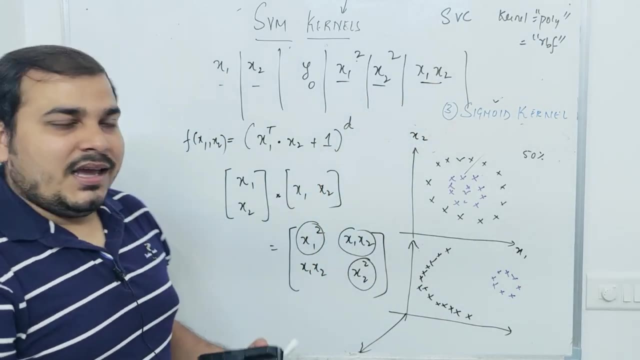 dimension. right, it will become that, looking like this in the polynomial form. now you may be thinking: Chris, how did it come right? you may be thinking because, just understand, we did X 1 square, X 2 square, X 1 and X 2, if you take this. 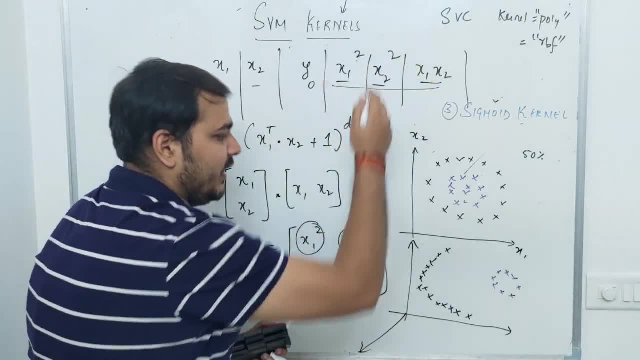 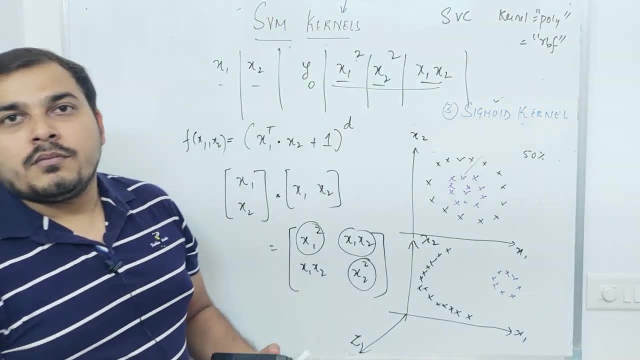 entire data set, this three data set, and plot it. it will be coming in this particular format. suppose this is my X 1, this is my X 2 and probably this is my Z right. so when I am taking this, this Z will be nothing but X 1 comma, X 2, X 1 multiplied by X 2. 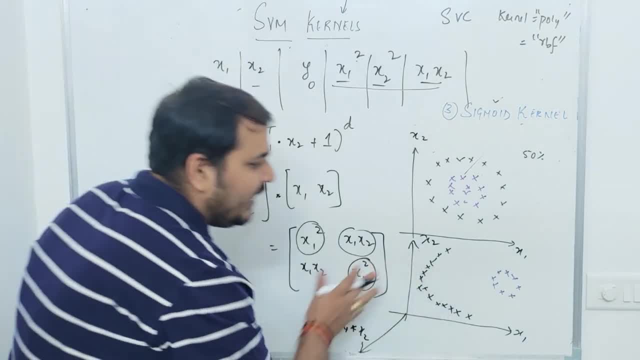 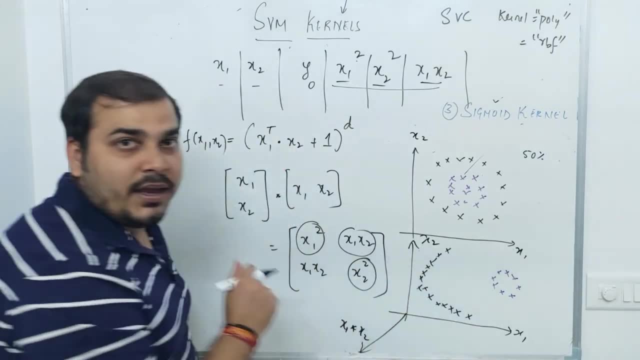 because X 1 multiplied by X 2 is nothing but this. now, when I try to plot this particular point, this will be looking like this and this will be having this polynomial shape. okay, probably the direction I put up will like this. it may be looking like that, but understand the direction can be. 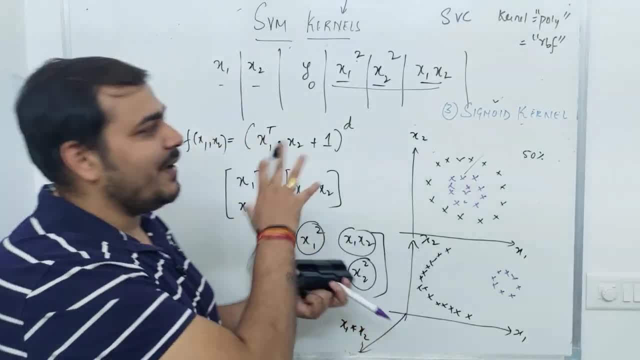 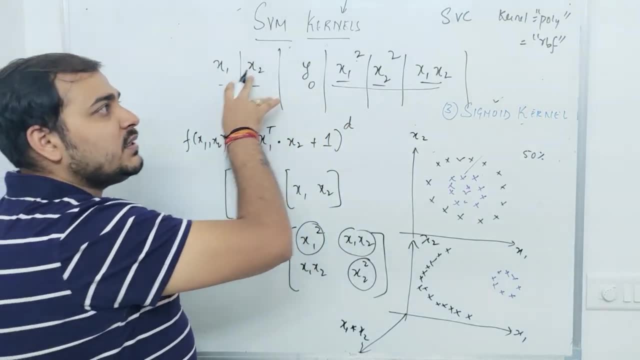 anything, it may be like this, it we like this because I'm not able to draw a three-dimensional over here for you. okay, just understand this. but here you understood right. initially I had two features. since I'm applying this polynomial kernel, what I did is I applied this polynomial kernel. what I did is I applied this polynomial kernel. what I did is I applied this polynomial kernel. what I did is: 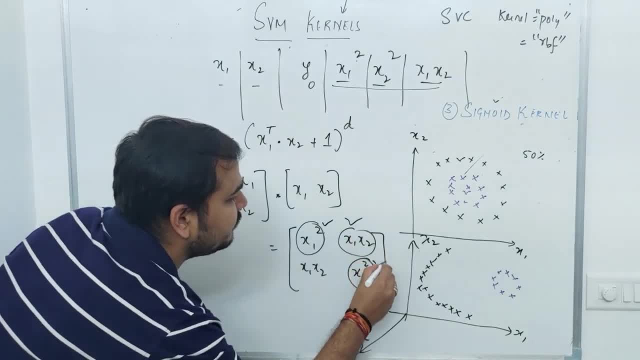 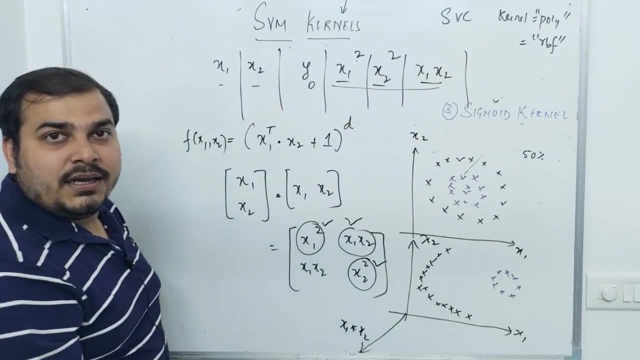 is that, based on this particular equation, I found out all the important components, right, and then I try to find out that specific data set over here. now, when I have all this particular data set, I saw the projection over here. now, don't you think we can create a straight line? 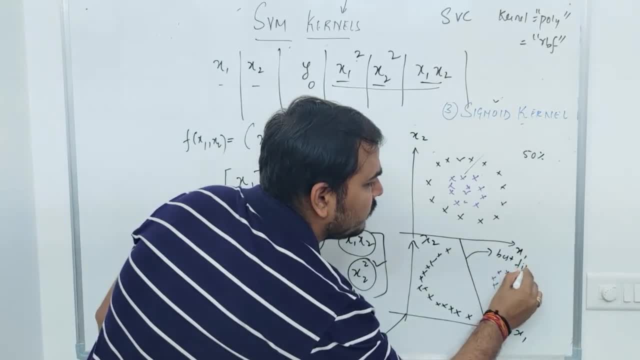 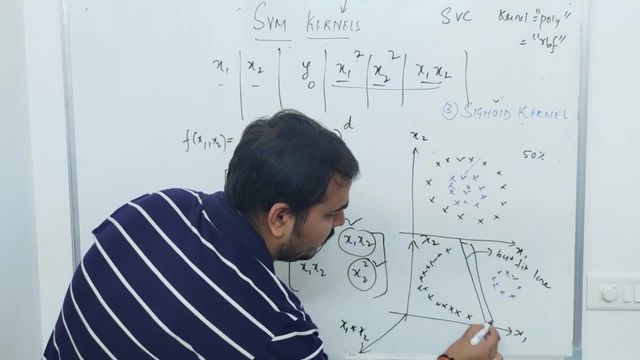 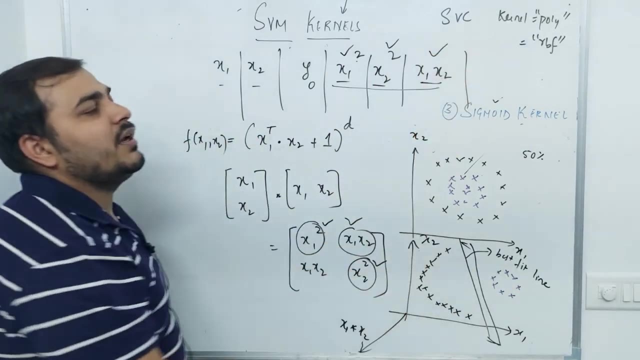 and this line will be my best fit line. this will be my best fit line in order to understand, in order to do the splitting. it will be like this kind of plane because, remember, this point that is getting plotted is nothing but x1 square, x2 square and x1 comma, x2, x1 multiplied. 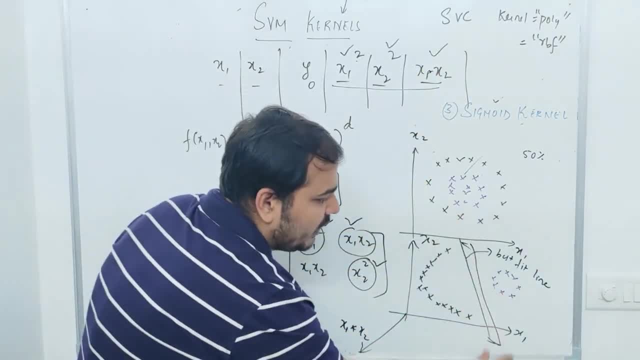 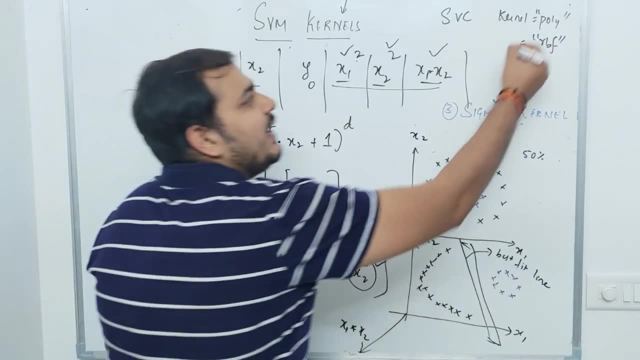 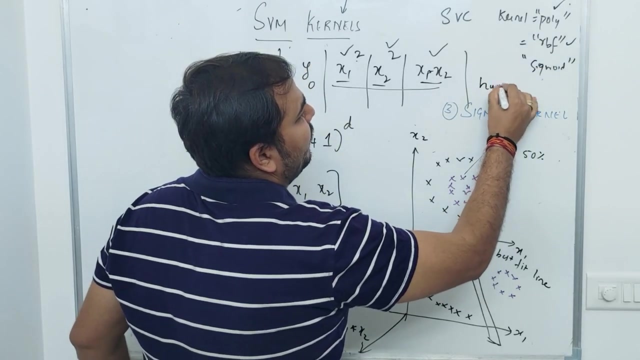 by x1, sorry. so now I will be able to create this plane line and basically do this kind of activity. now the thing is that how do you decide whether we should use polynomial rbf or sigmoid? this is purely determined by, which is called as hyperparameter tuning. see, guys, 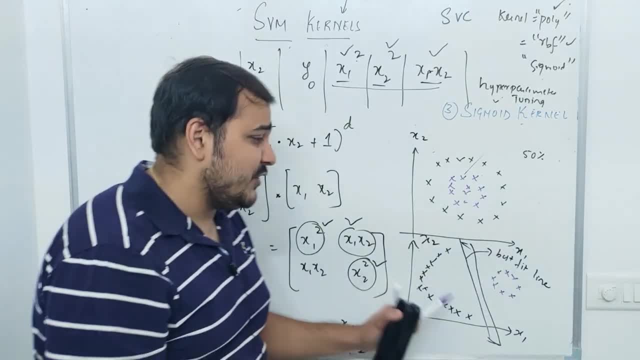 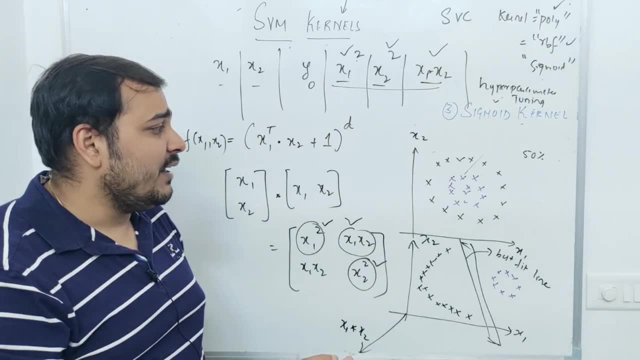 you may getting confused because I probably did not show you the hyperparameter tuning. I will show you any kind of visualization with the help of code. my next video will be about that only, and there you will love it. and trust me, you will be loving it because 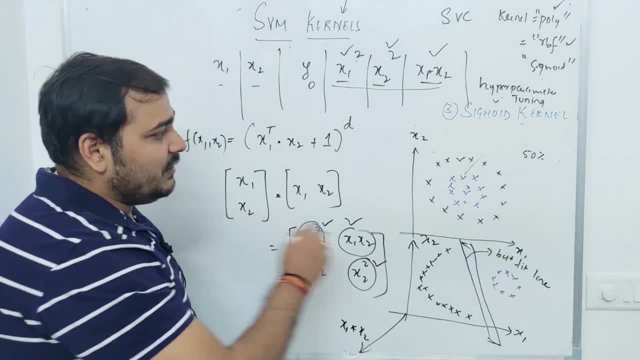 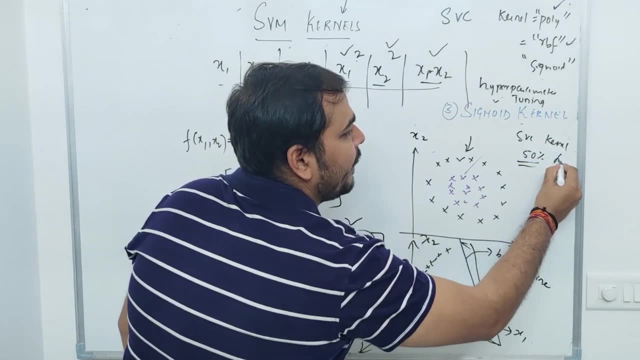 I will be having similar kind of data set and suppose I plot this kind of data set over there. I try to apply a SVC with kernel linear. suppose I am using a kernel linear. that basically means I will try to draw a best fit line here. you will be getting an accuracy of somewhere. 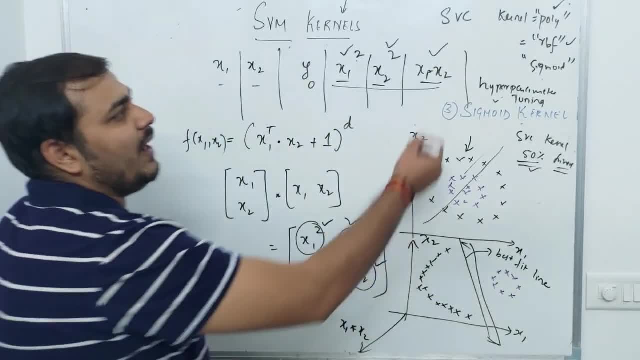 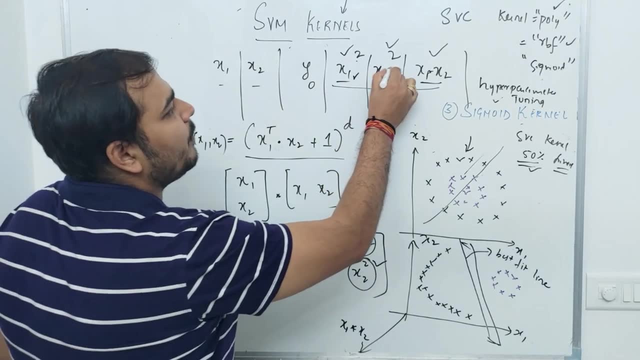 around 50 percent. so after that, what I do is that I apply a polynomial rbf and then I will draw a polynomial kernel in polynomial kernel. I need to apply this particular operation and, based on this particular operation, I need to find out these all components now once. 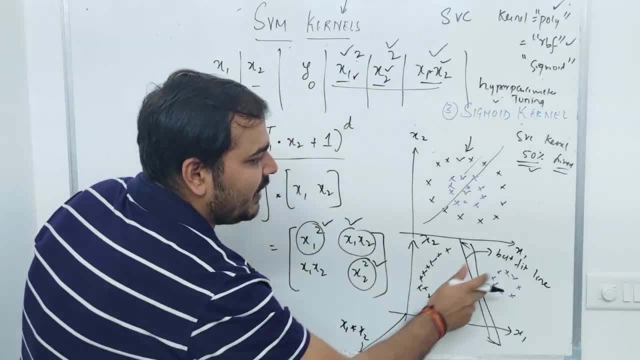 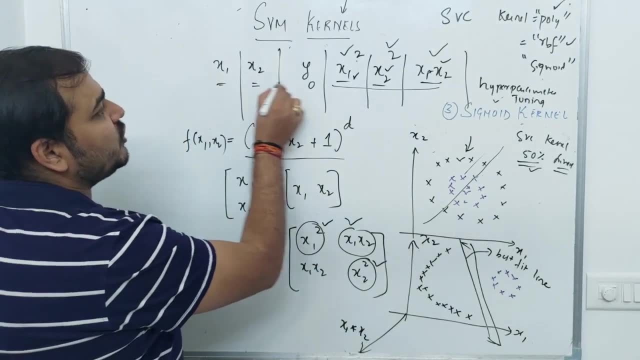 I got all these components. if I try to project this now, my data set will be looking like this right in the three dimension. before this, I can also use x1, x2 and probably this particular parameter. there you will be seeing that the data will be too much intermixed, but if I 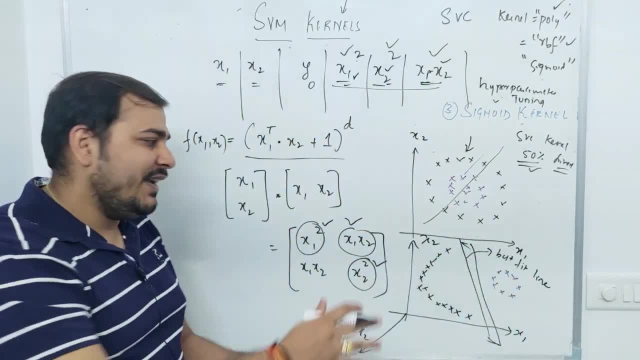 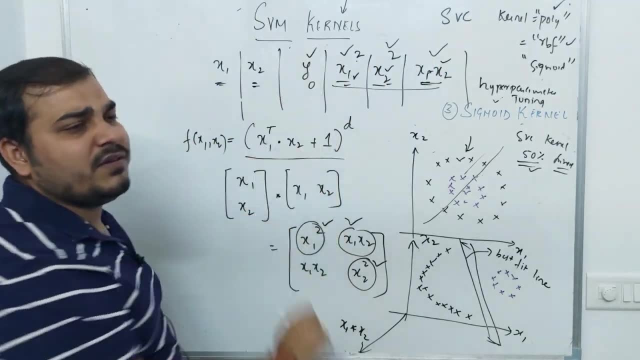 just use this values and probably plot it here, you will be getting a higher dimension data set. Now see, initially I have two features, now I have three features and obviously this is my output feature. this is for my marking of that particular class 1 or class 2. now when 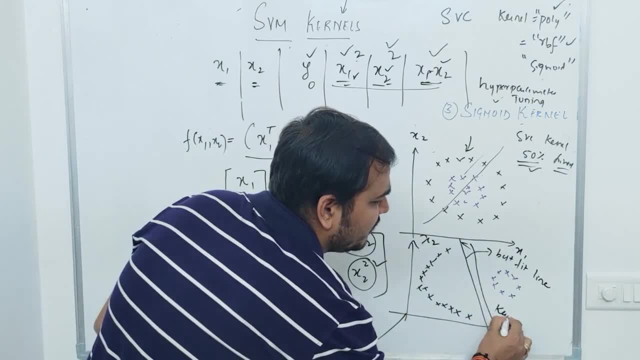 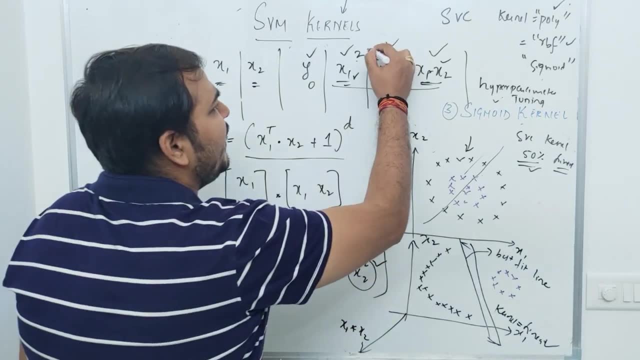 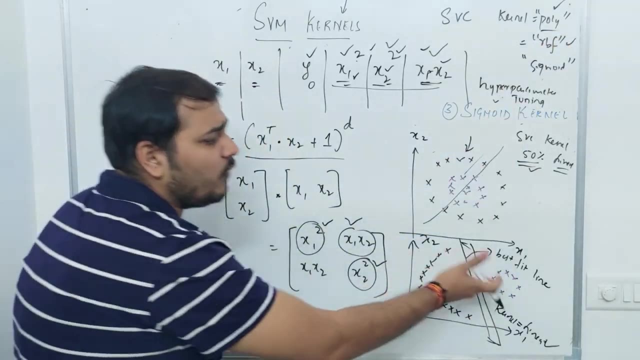 I draw this now. once I get this, I can definitely use my kernel is equal to linear and probably create a plane. now you may be thinking: krish, why did we do this? instead, you could directly say kernel as poly or kernel as rbf and you could have directly found out this particular